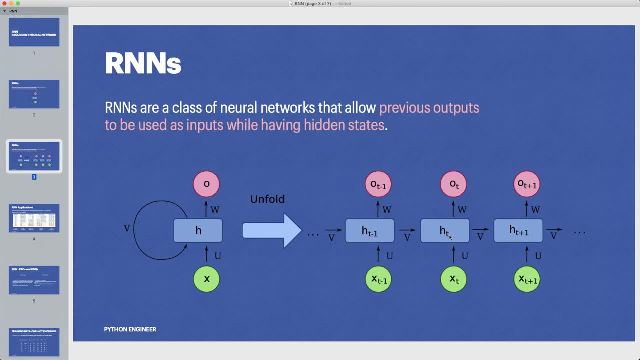 And then we use this hidden state and then put it into the next input. So we take the next input and use the previous hidden states and again do our operations and get a new output and then new, updated hidden state, And then we take the next input and so on. 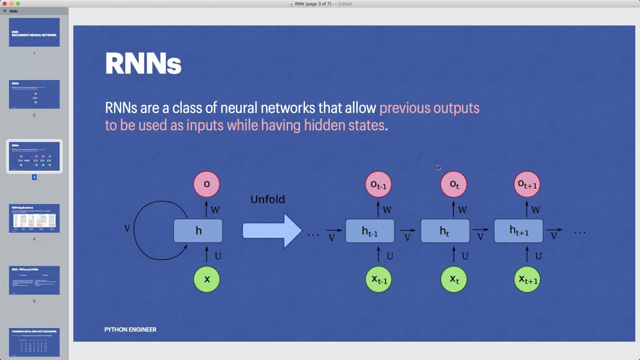 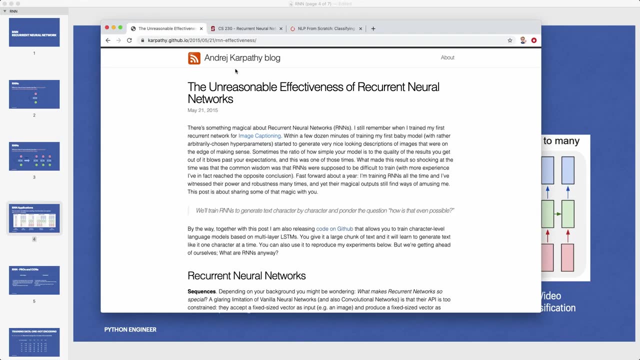 So this is basically the architecture of an RNN. And now why aren't aren't so important? And for this there is a new state which is called the DarkSenseAtol, And this is the storage state, which is nice. article by Andrej Karpathy. The article is called the unreasonable- unreasonable effectiveness. 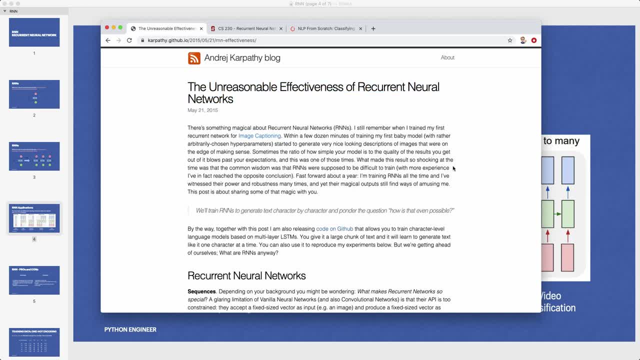 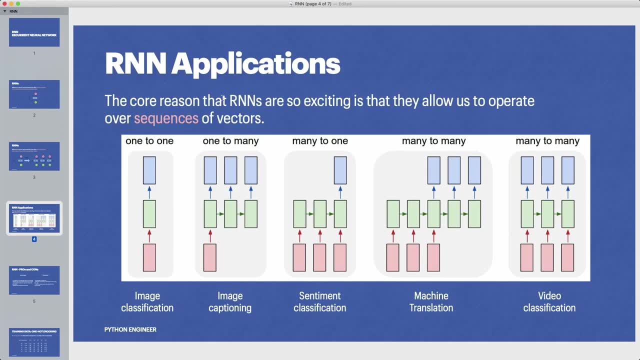 of recurrent neural networks And I highly recommend to give this a read. So I will put the link in the description. But the core takeaway is that RNNs are so exciting because they allow us to operate over sequences of vectors. So with traditional neural nets we have just a one to one. 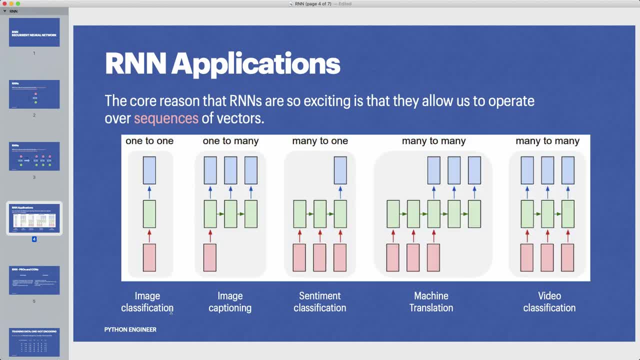 relationship. for example, when we do image classification, then our input, so our image is a fixed length and our also, our output is a fixed length. And now with RNNs we can work with sequences And there are a lot of different types. So basically we can have a sequence in our input. 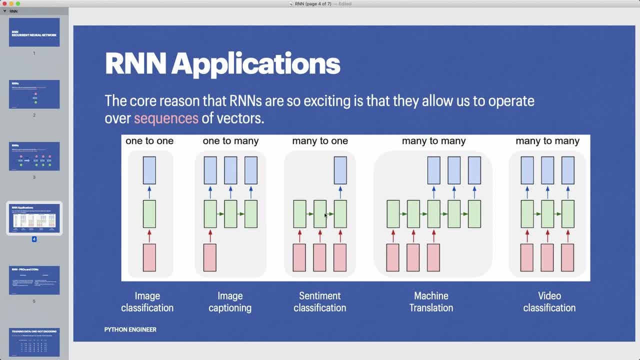 and we can also have a sequence in our output or also in both inputs. And we can also have a sequence in our output or also in both inputs And output. So, for example, we can have a one to many relationship where we have only one input. 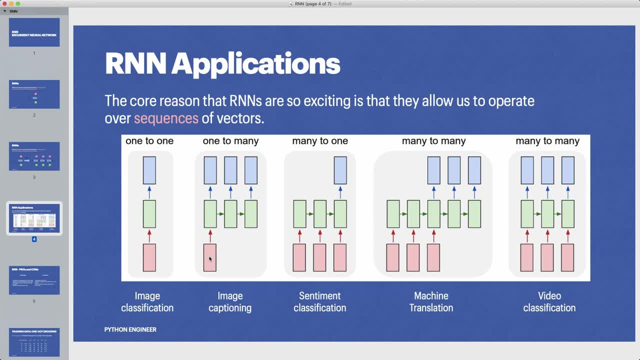 for example, this is used in image captioning. when we have one in image and then we want to describe what we see in the image and get multiple outputs, then we can also have a many to one relationship. So we have. this is, for example, the case in sentiment classification or what we are. 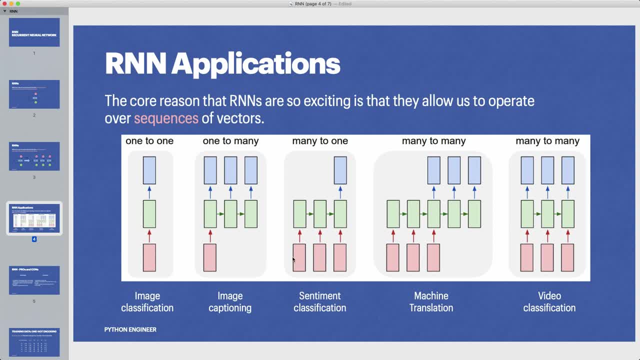 doing later. we can also have a many to one relationship. So we have- this is, for example, the case in sentiment classification or what we are doing later with our name classification. So we have a sequence as inputs and then apply our RNN And then we use the last. 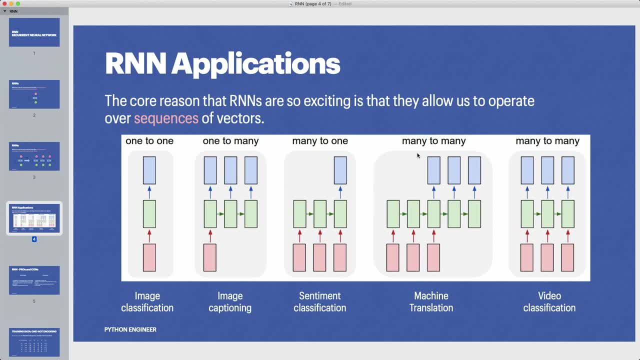 output and do some classification with this, then we can also have a many to many relationship. This is, for example, used in machine translation, where we have a whole sentence, for example in English, as an input And then we put out a whole sentence in French, for example. 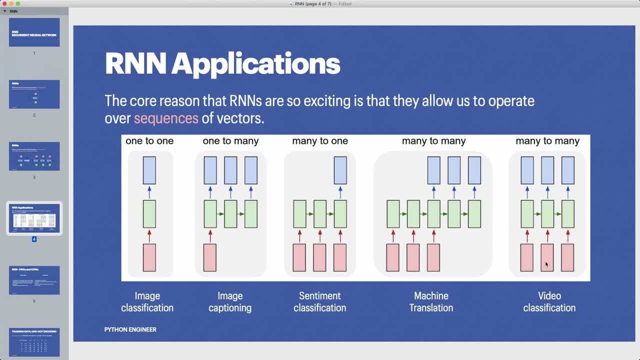 Then we can also have a many to many in relationship with a synced way, for example in video classification, where we want to classify each single frame. So yeah, these are our possible applications of RNNs. So they are mostly used in the fields of: 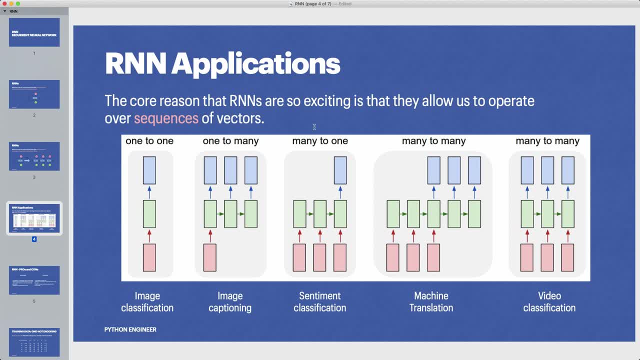 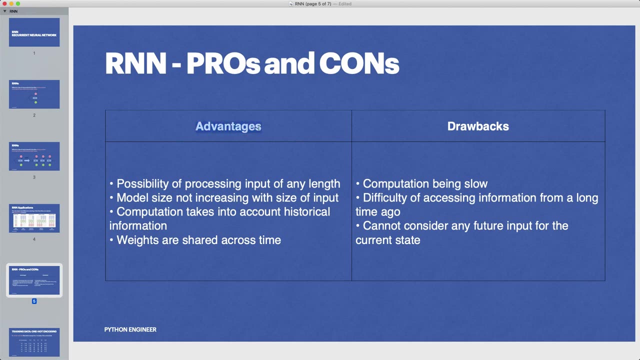 natural language processing and speech recognition, But they could, for example, also used for image classification. So, yeah, that's what makes RNN so powerful. And now let's have a brief look at some pros and cons. So the advantages are that we have 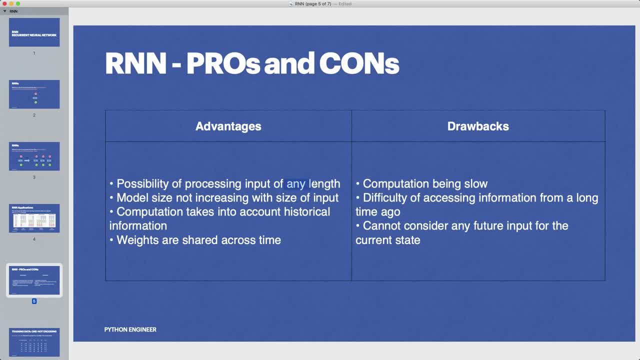 the possibility of processing inputs of any length. then our model size is not increasing with the size of the input. then the computation takes into account historical information. So the previous data and our weights are shared across time. And some drawbacks are that the computation might be slower than with normal neural nets And it can be difficult. 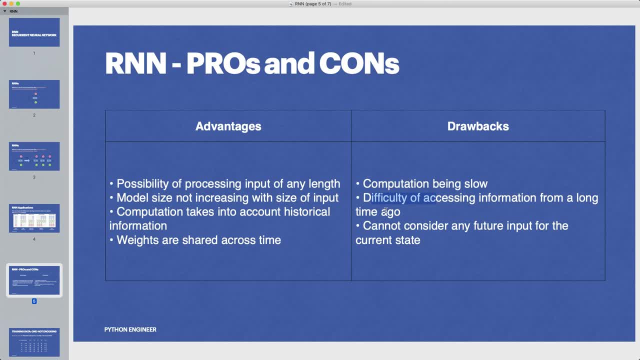 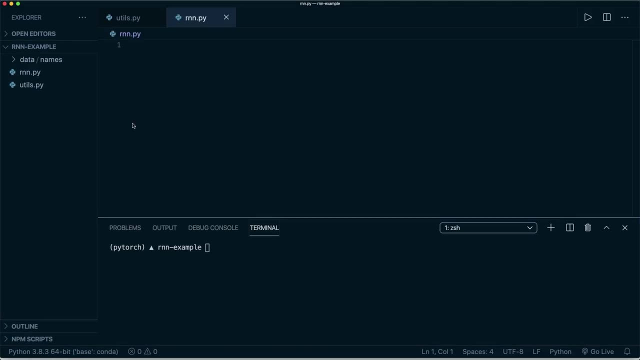 to access information from a long time ago And we are also not able to consider any future input for the current state. So yeah, that's basically the theory behind RNNs And now we can directly jump to the code. So in our example, we want to do name classifications. 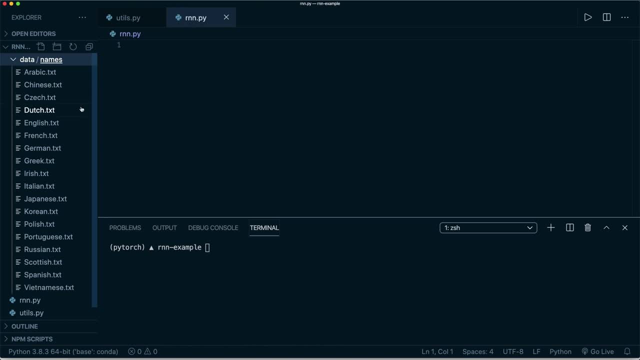 So I downloaded the data and I will also put the link in the description. So basically, we have different files with different names. So these are all last names from different countries. For example, we have Arabic, Chinese, Czech, Dutch, English and so on. So I think 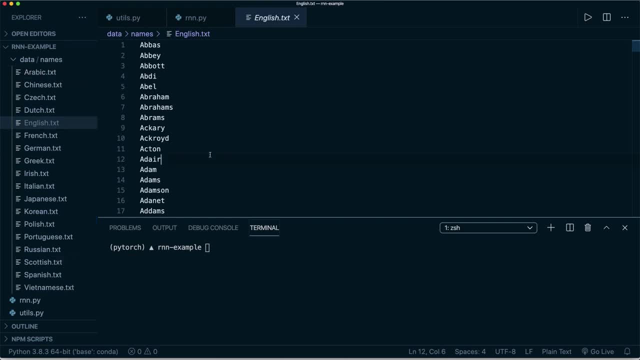 these are 18 different countries. And now we, what we want to do is we want to create this, we want to classify this and detect from which country the name is, And what we're going to do here is we take the whole name as a sequence And then we use each single. 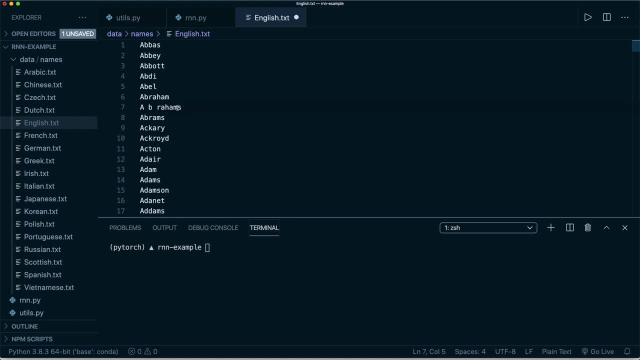 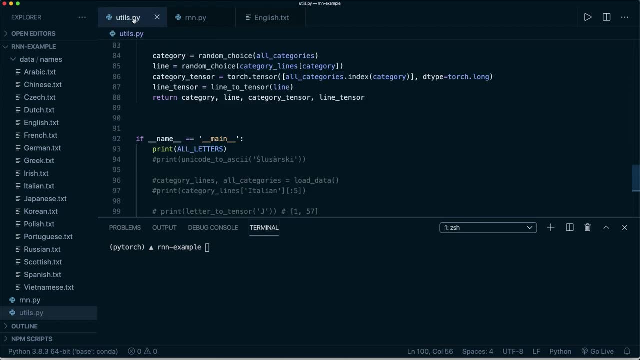 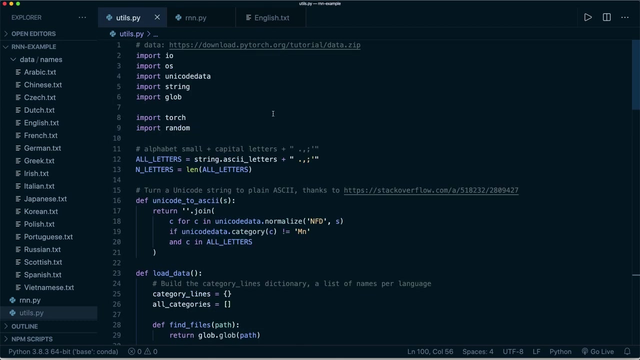 letter and put it in our RNN as one input, And for this we need some helper functions. So I already Implement, Okay, presented them here, And I will only go briefly through this code. So what we want to do here. 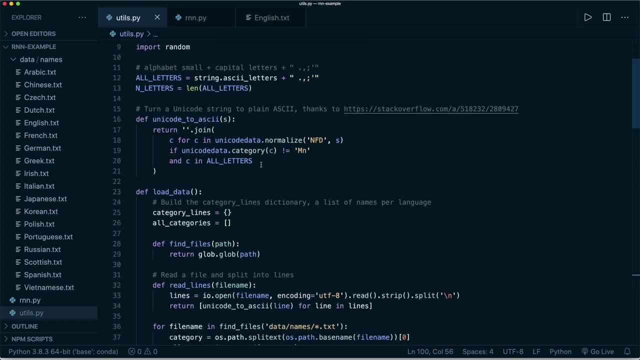 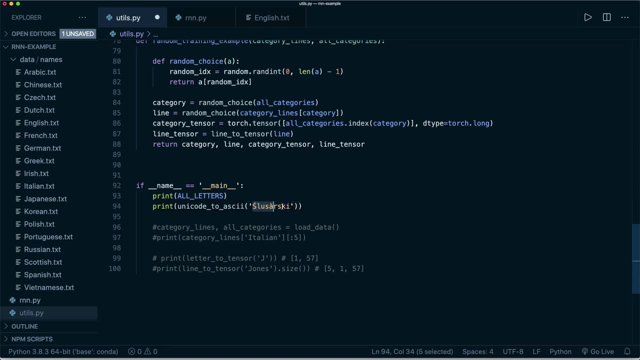 first, we want to have a helper function to convert our data to ASCII. For example, if we have this name with some special characters and then we process this, so let's run this file, then we see it remove the special characters and we only have ASCII characters left, And 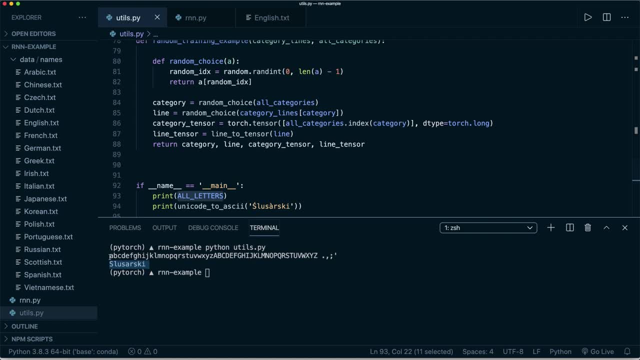 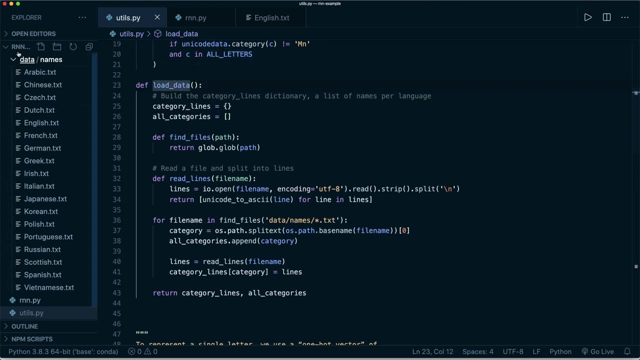 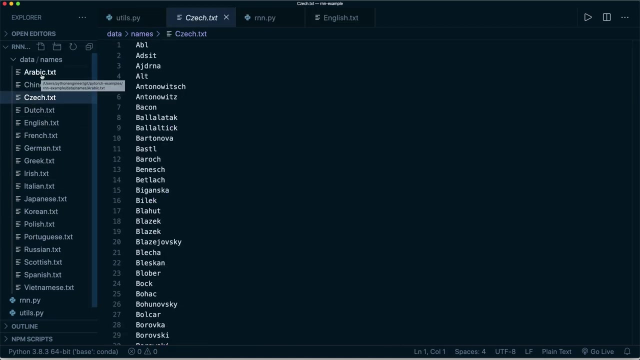 basically we also print all the possible letters, So this is from A to C and also in capital letters And we also allow these signs. And then we have a helper function to load the data. So this basically loads all the those files And then it loads all the names and it gets the country from the file name. 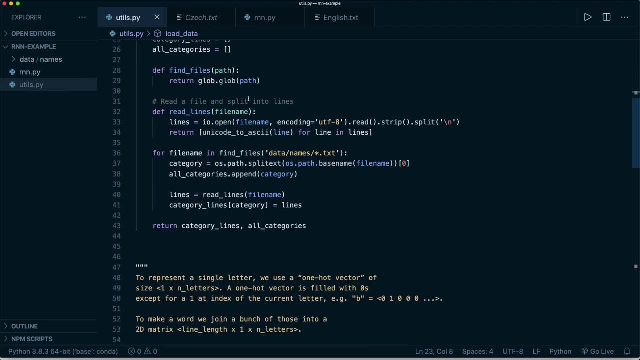 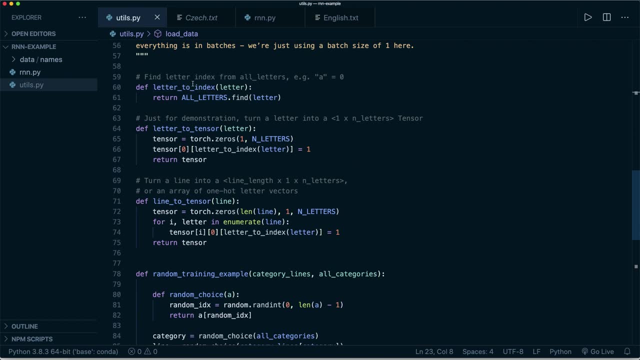 So this is what the load data function will do, And then we have some functions to turn our data to tensor. So we have letter to index and letter to tensor and also a line to a tensor. And what we are doing here is we are using a technique that is called one hot encoding. 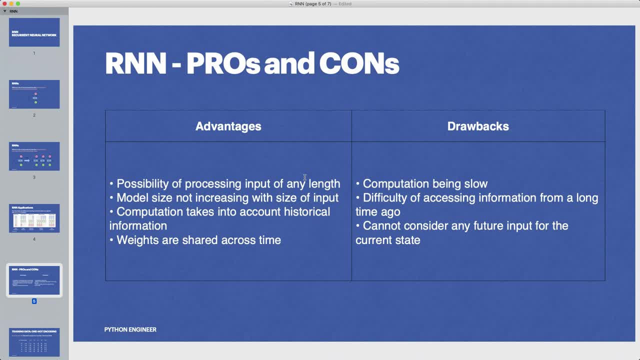 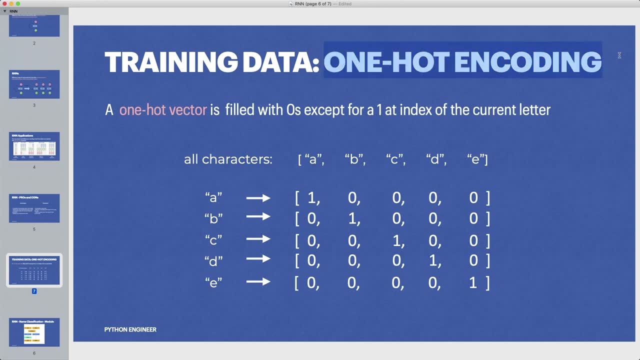 So we need a way to display our data And that can be used for training, And for this we use one hot encoding. So if you've watched my tutorial about the chatbot in pytorch then you might already know this. So a one hot bed vector is filled. 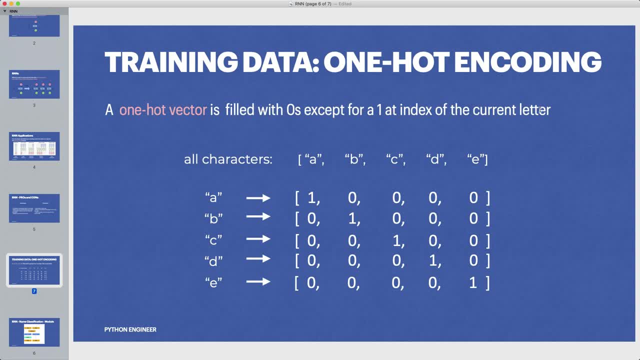 So a one hot bed vector is filled. So a one hot bed vector is filled with zeros, except for a one. at the index of the current letter, For example, if we have only five possible characters- a, b, c, d and e- then our a would be a vector of length. 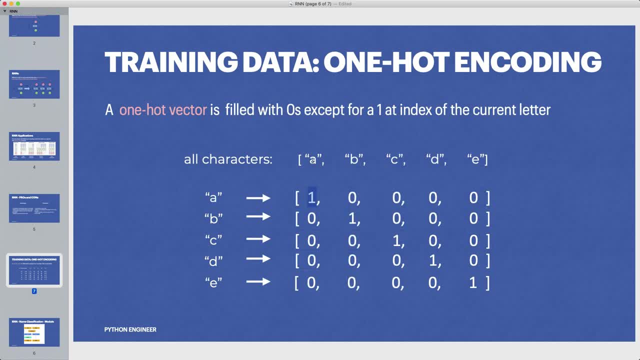 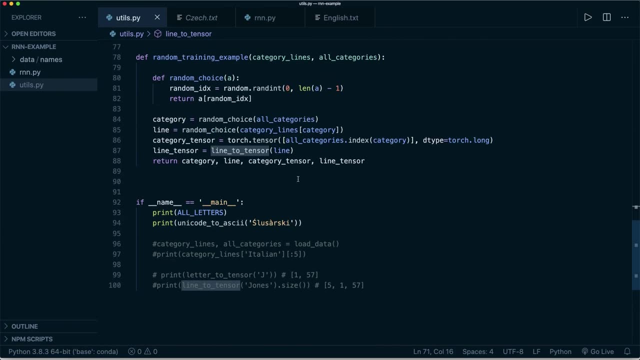 five, and we have a one at the position where a is, and the same for B, a vector of length five, and the second index is a one and the rest zeros. So this is one hot encoding. So this is one hot encoding. So if we go back to our file, for example, I can show you. 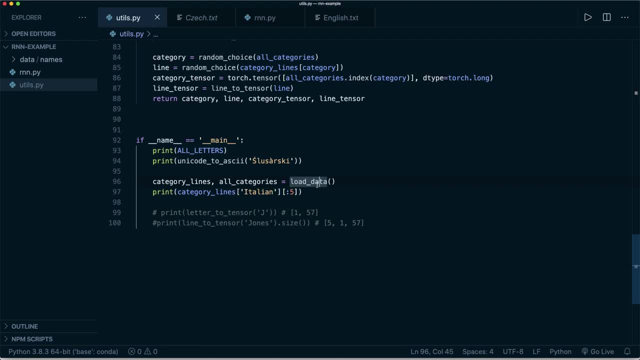 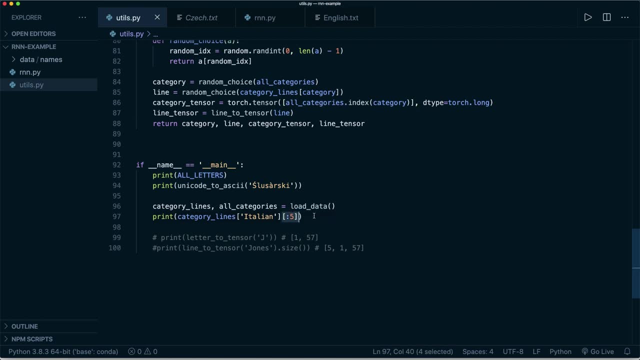 how the loads data function looks. So this will return a dictionary with the country as key and then the corresponding names as the values. So, for example, if we run this and have a look at the key Italian and only take the first five entries, then we see that. 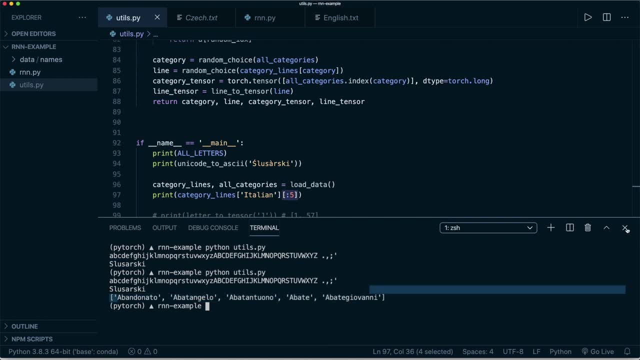 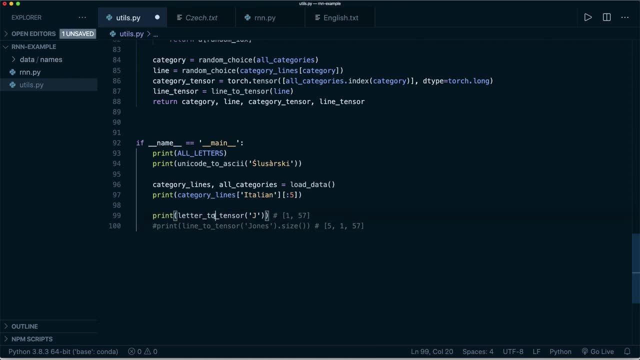 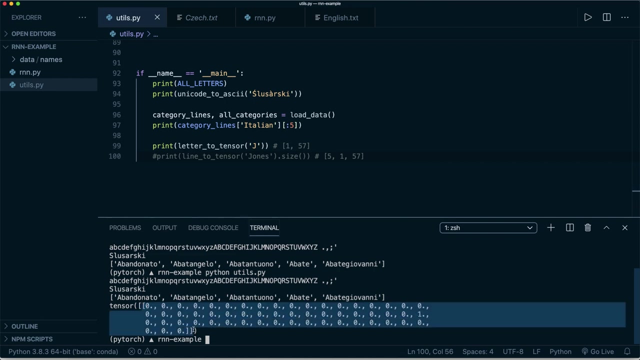 we have five different Italian names here. Then, as I said, we do this one hot encoding, So for this we can use the letter to tensor function. So now if we run this, so let's save this and run this, and then print the tensor for J, then we see it has this size. 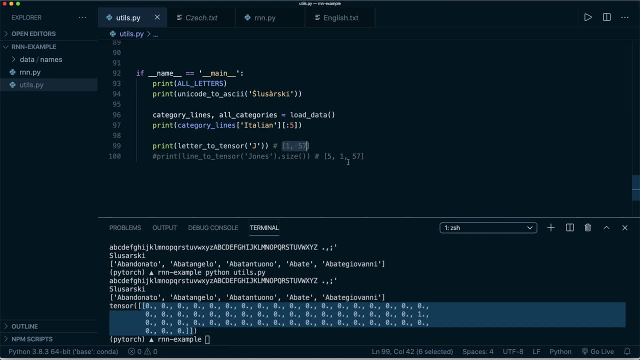 So this is of shape one by 57. Because we have 50 of them, 57 possible characters. this is what I printed here. these are all the letters, And then we have a J at the position where the capital J is. So this is how our input will look like. 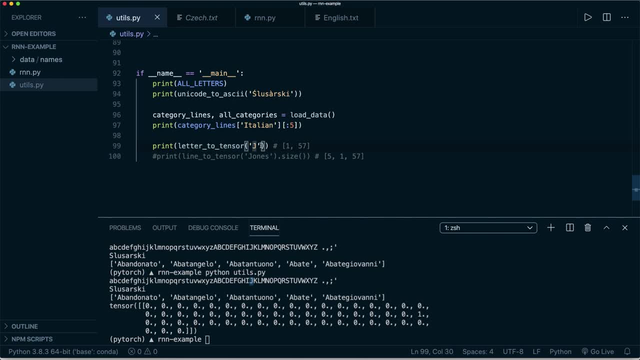 like later. And of course we do this not only for a single character but for the whole name. So for this we have the line to tensor function And now if we here, we print the size, so this will be of size five by one by 57. And 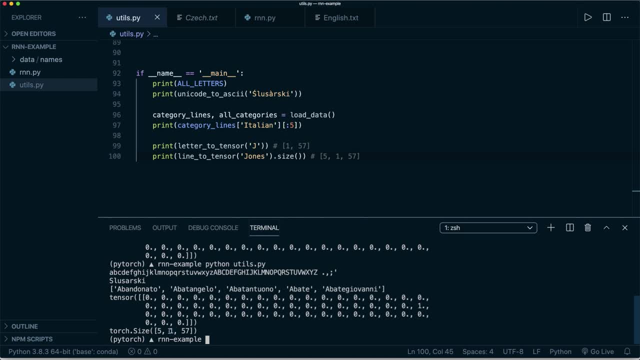 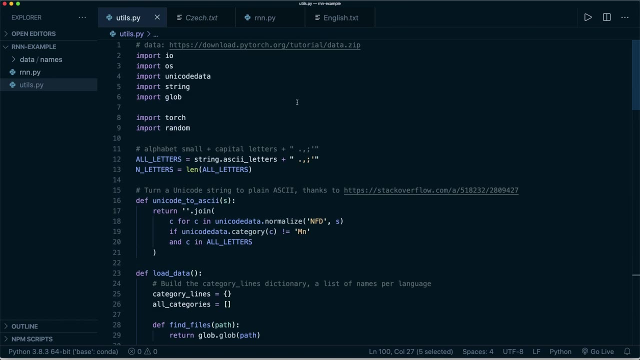 the one is because our model expects it to be in this shape, And the five is because of the number of characters and the 57 is because of the number of all different characters. Alright, so these are all the helper functions that we need And, of course, I will put the 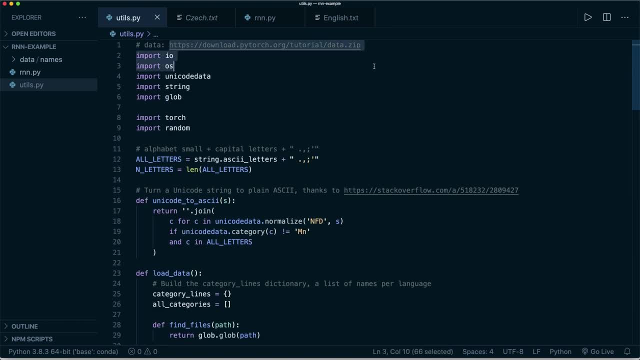 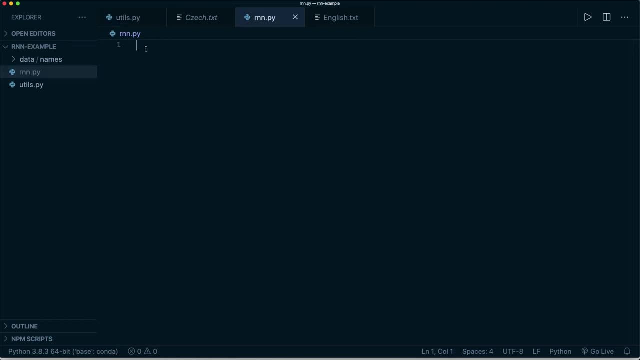 code on GitHub And I also provide the link to the data so you can download these files. So now we can start writing our RNN. So for this, of course, we import the things we need. So we import torch, we import torch dots, n, n, s, n, n. then I will also want to import mat, plot, lib dot. 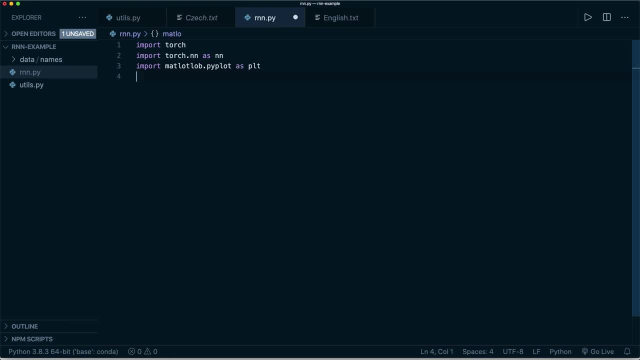 pi plot as PLT, Because I want to show you a plot later met plot lip. then we import our utility functions. So I say from utils, import all the different letters and also the number of different letters. So this is 57. Then we also say from utils we want to import these helper functions. 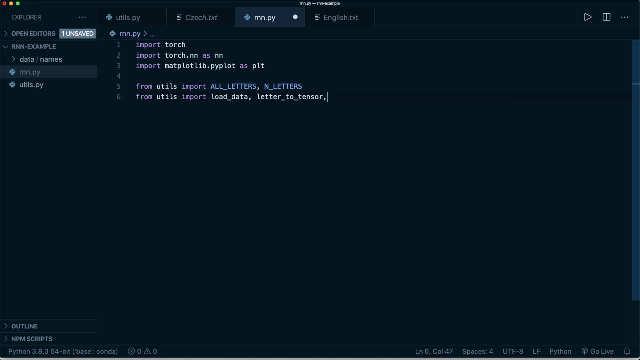 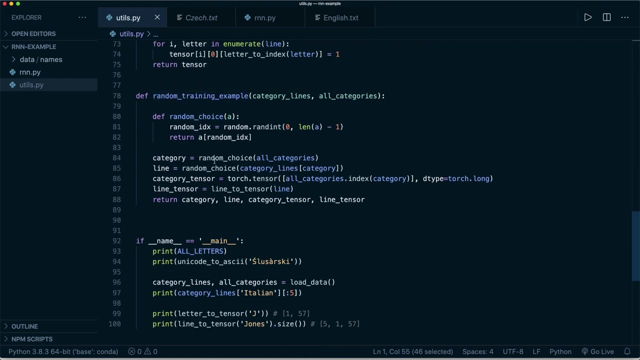 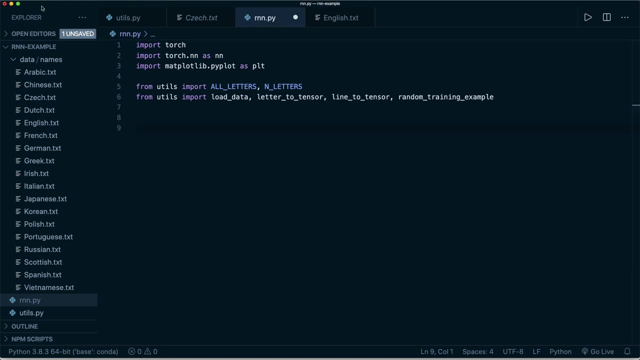 So load data, then left to tensor and line to tensor and random trainings example. So this is basically a function that will do a random choice from those names and return the corresponding country. So now that we have that, we can start implementing. 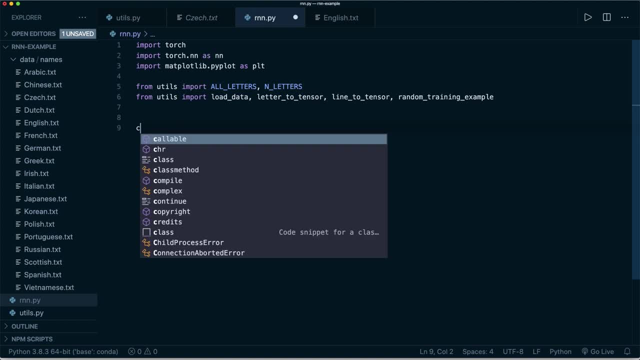 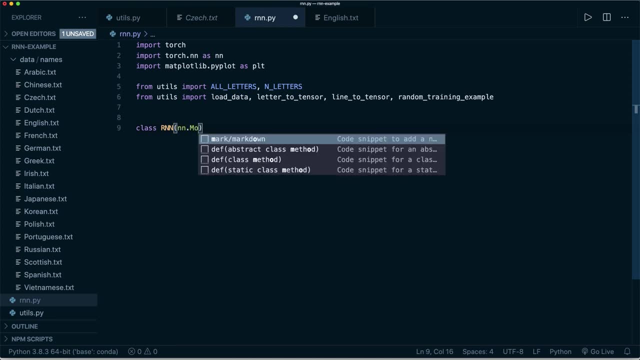 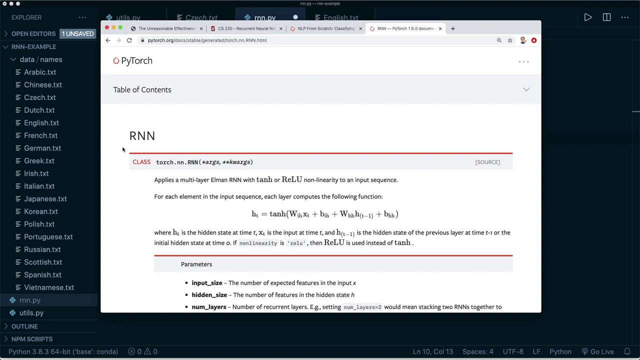 our RNN. So we need to have a class and call this RNN And this should inherit from n n dot module, as all of our pytorch models. And, by the way, there is already a RNN module available in pytorch So you can directly use this. but this is what we are doing in. 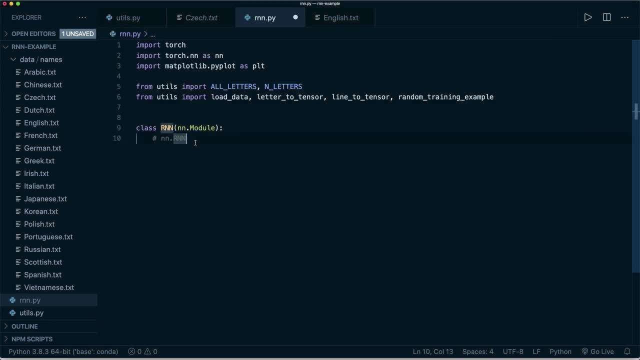 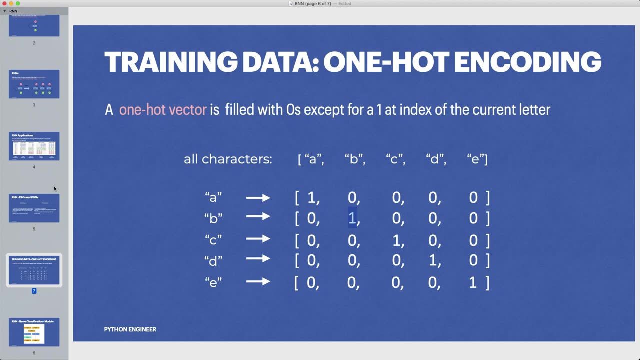 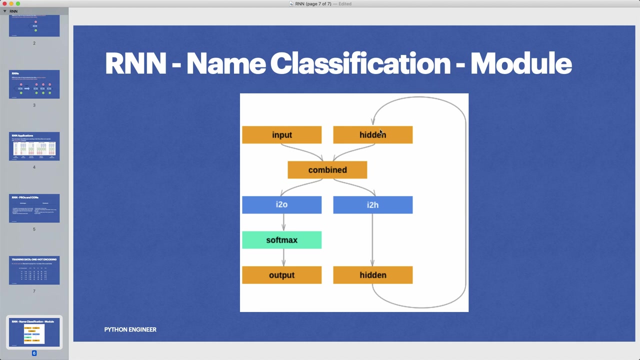 the next tutorial. So for now, we want to implement this from scratch to get a better understanding. So let's have a look at our model architecture again. So this is what our RNN for name classification will look like. So we have an input and a hidden state And then internally, so this: 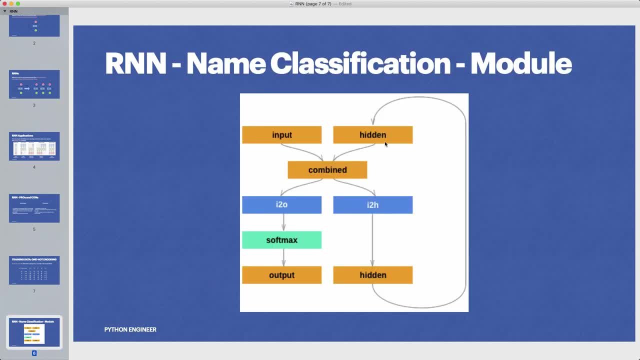 is what we are doing here internally. So we combine them and then we process our combined tensor and we apply two different hidden layers. So we have our input to a output and our input to a hidden layer. So these are just two normal linear layers And then we get one hidden output and then we use this. 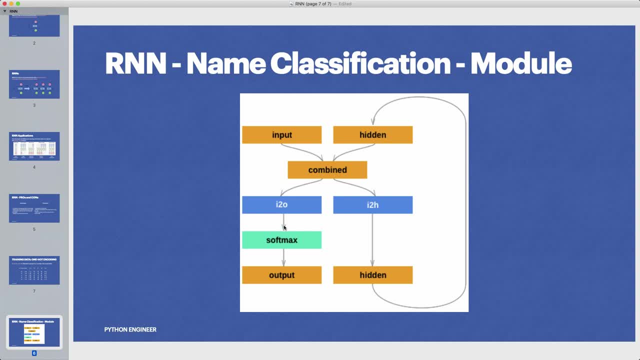 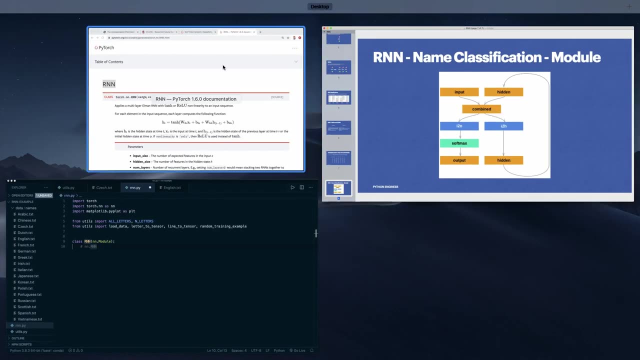 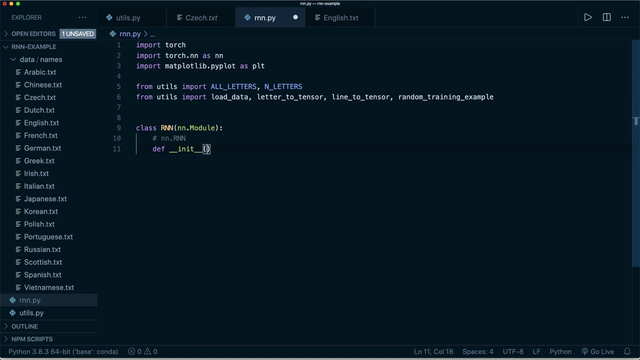 for the next input And we also get a output. And since we are doing classification, so a multi class classification task, we apply this softmax layer and then get the output. So now, this is what we want to implement. So now, first of all, of course, we define our init function. this will get self. then 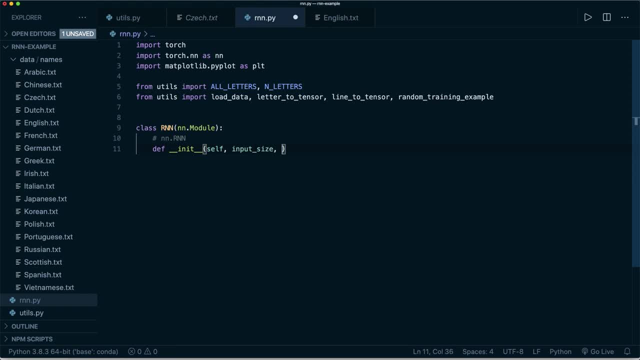 it gets the input size, also gets the hidden size. So this is going to be a hyper parameter that we can specify, And we also get the output size. And in our init function first we want to call this super RNN and self, and then 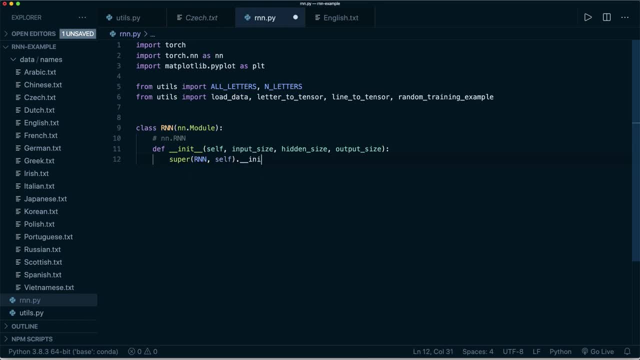 the in, it's sorry in it. Then here we want to store our hidden size, so we say self dot, hidden size equals hidden size. then we define our two different linear layers. So we call this input to hidden. i to h equals nn dot linear And the size is the input size plus the hidden size. because 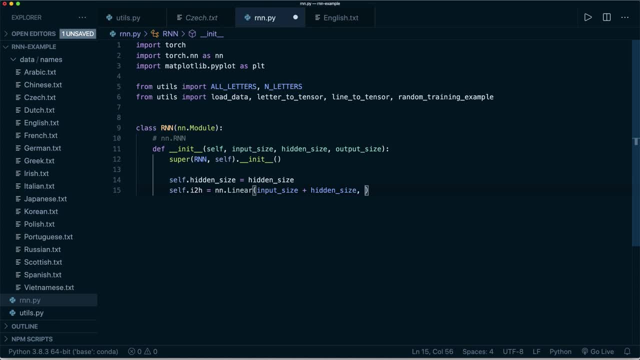 we combine them, And for this the output size is still the hidden size. then we do the same with our output. So we say input to output, and this is going to be a linear layer as well. So the input size is the same, And here we use the output size. And then 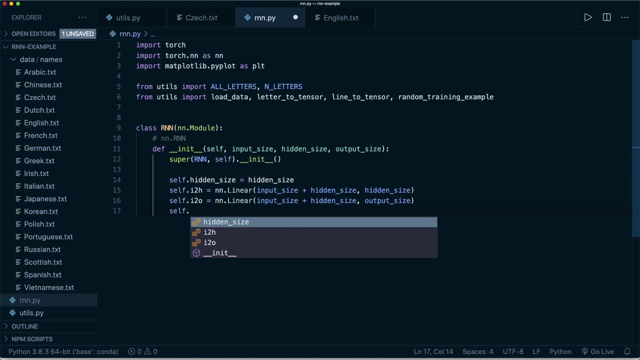 we also need a softmax layer. So we say self dot soft max equals nn dot lock soft max. And then we say that dimension equals along dimension one, because our input, for example, just test the shape one by 57.. So we need the second dimension. So this is our init function. then we of course 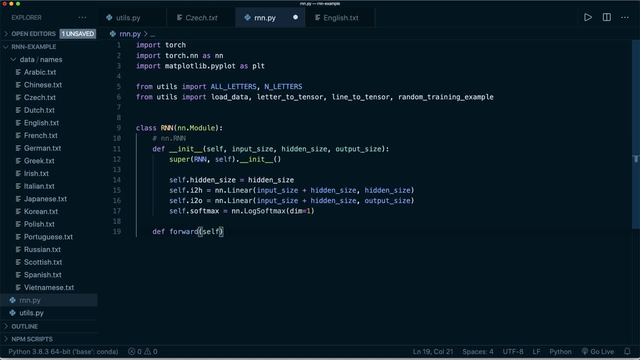 also have to define the forward pass. So we say, define the forward function and this gets self, and then it gets an input tensor And, as you should know, now this also gets the hidden tensor. So we use the hidden tensor for the forward pass, And then here we process this. So first, 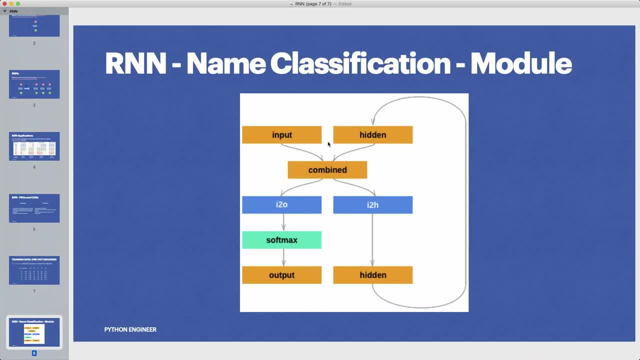 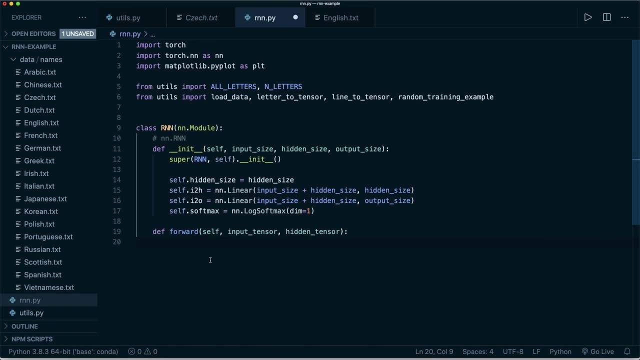 thing. let's have a look at this again. we combine our input and our hidden tensor and then we apply those linear layers and the softmax And then we return to different tensors, So the output tensor and the new hidden tensor. So let's do this, So let's call this combined. 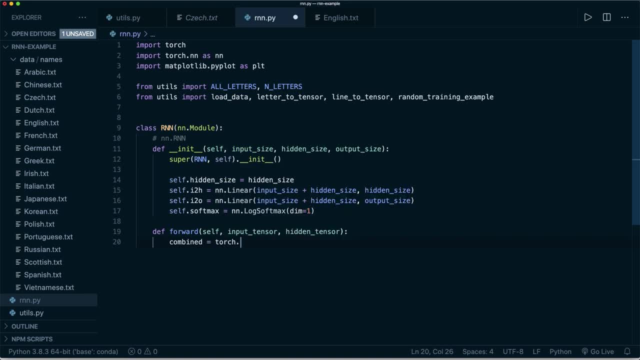 equals. for this we can use torch dot cats, And then as a tuple we want to combine the input tensor and the hidden tensor, And here again along dimension one, then we apply our linear layers, So we say hidden equals, self dot i to h, And then here we put in the combined tensor, then we say our output. 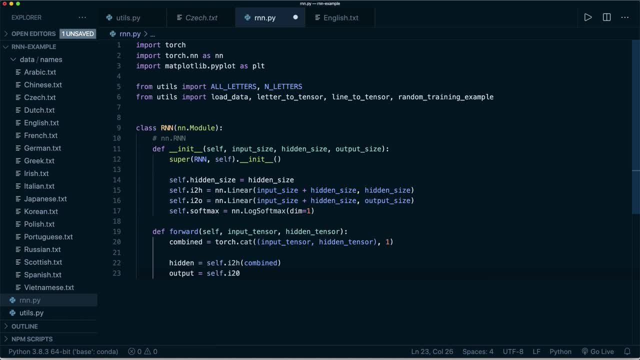 equals self dot i to o o with our combined tensor as well, And for the output we also apply the softmax. So we say output equals self dot softmax with the output, And at the end we return the output first and then the new hidden state, And so this is basically all we need for our 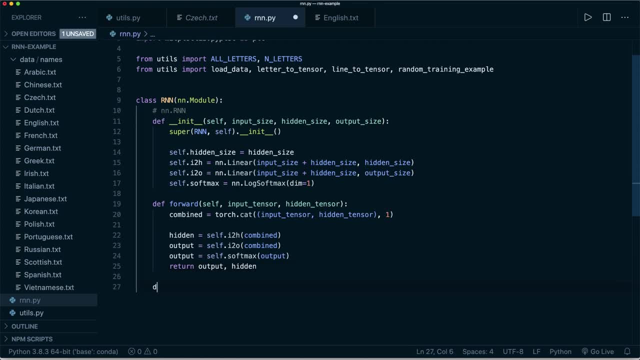 RNN Implementation And I'm also going to add a new, a little helper function And I call this in it hidden. So I need some initial hidden state in the beginning And what I want to do here simply is I want to return an empty tensor. So I say torch dot zeros And this has the shape: one by self dot. 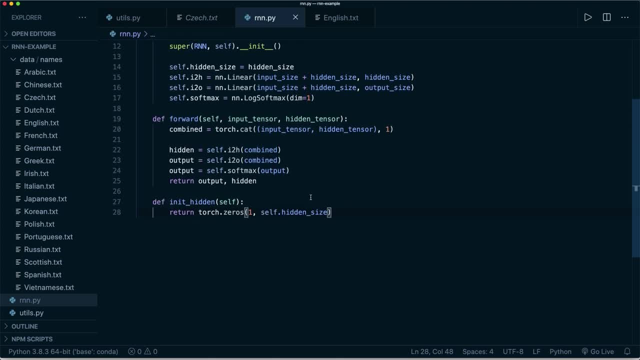 hidden size And yeah. so now we can start applying this. So now let's load the data. So let's say, our category lines and our all possible categories equals load data. So this is a dictionary with the country as key and the names as values, And this is just a list of all the different. 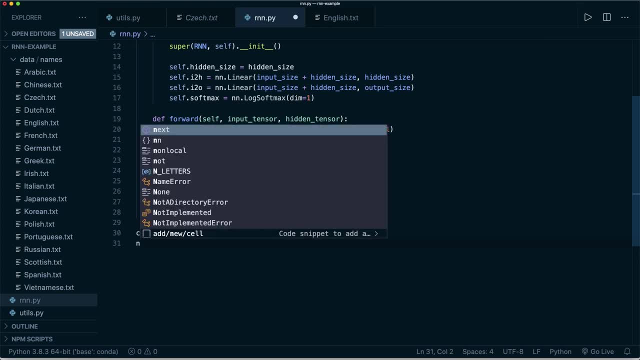 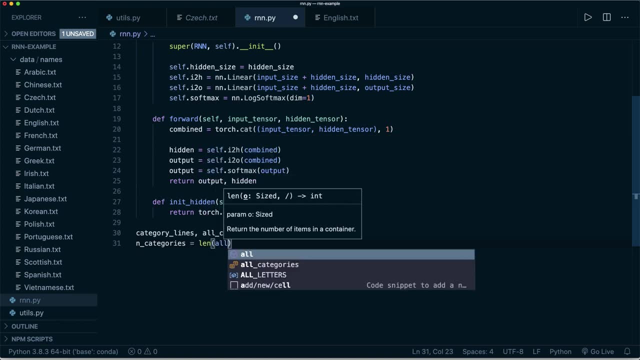 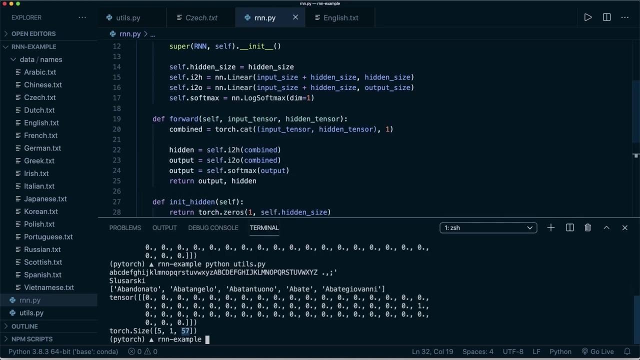 countries, And then the number of categories equals the length of all categories. For example, we can print the number of categories And let's save this for now and see if everything is working. So let's say Python, RNN, dot, pi, And now this is working. So we see we have. 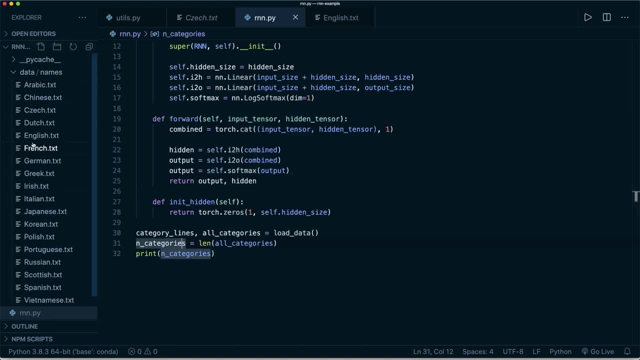 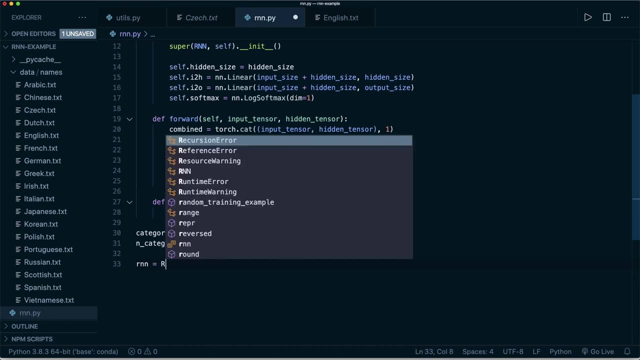 18 different categories. So this is because we have 18 different files here, And now we need to define or set up our RNN. So we say RNN equals and then we use our RNN class and this gets the input size, which is the number of possible letters. then it needs the hidden. 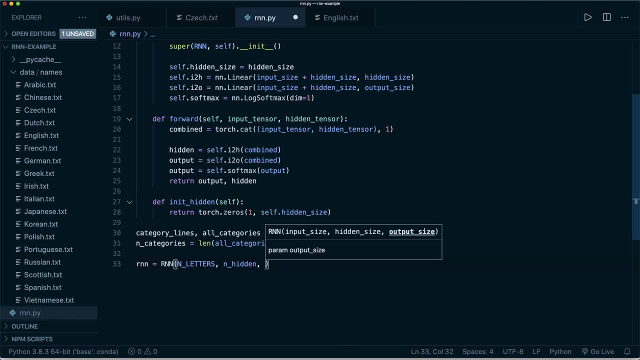 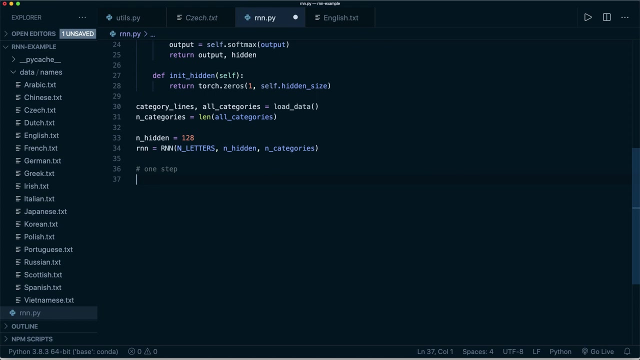 size, So, and hidden, and it needs the output size, And this is the number of categories. And now our hidden size. So, and hidden is an hyper parameter that we can define. So here let's try 128.. And now, as an example, let's do one single step So we can, for example, say our: 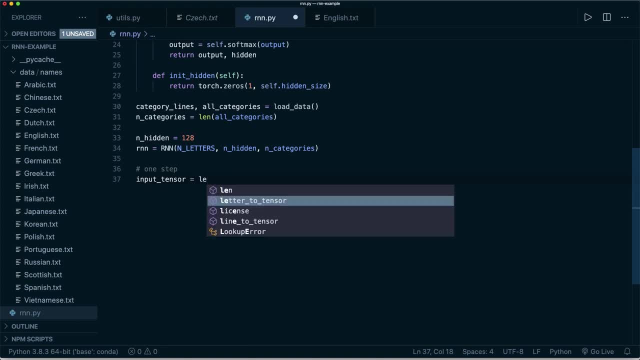 input: tensor equals, equals, and then we use the letter to tensor function for, let's say, for a and our. then we need a hidden Lakshmananer version, So hidden tensor equals, RNN, dot in it guiding, And then we process this, So we say output and then X. 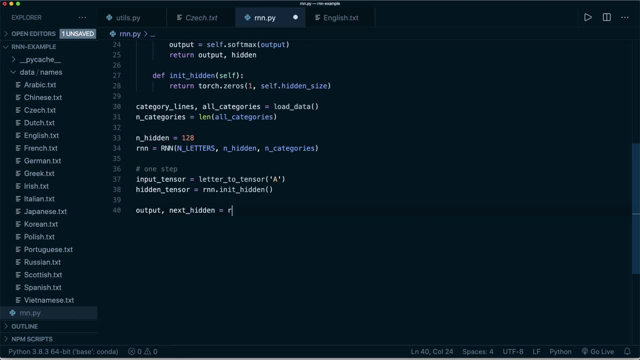 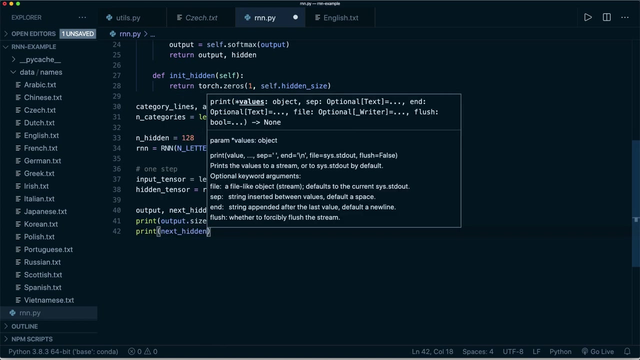 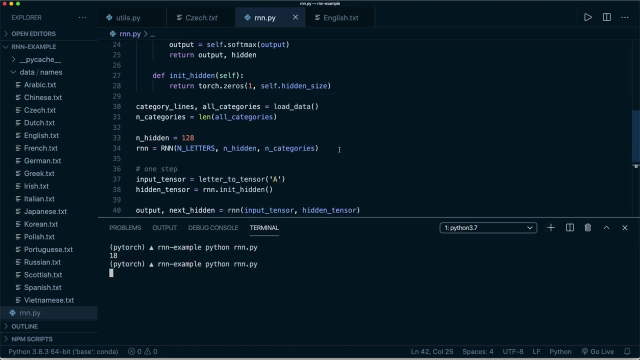 hidden equals RNN n with the input tensor and the initial hidden tensor. And now, for example, we could print the output size or shape. And let's also print the next hidden shape or size And let's run this and see if this is working. So yeah, we see our n RNN applied, the forward pass. 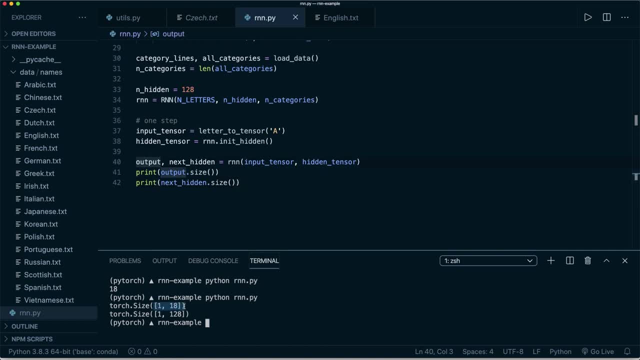 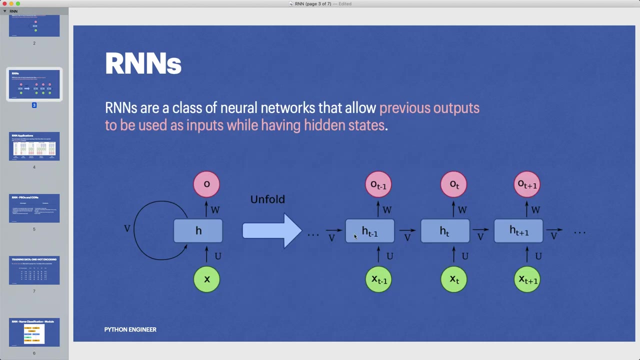 and we get the new output with this shape and a new hidden state with this shape. So it's still the size of the defined hidden size. So this is how it works for only one character, And now if we go back. so now, basically, we want to treat our 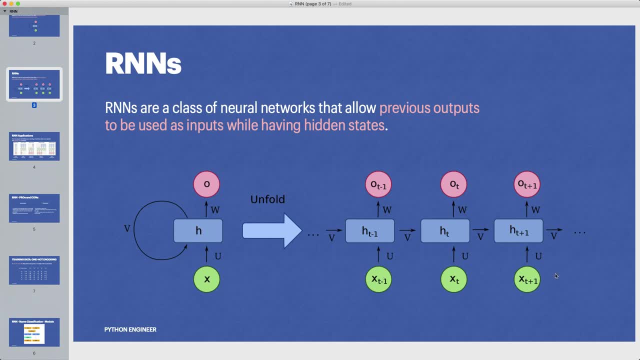 our name as one sequence and then each single character is one input. So we repeatedly apply the RNNs for all the characters in the name And then at the very end, we take the last output and apply the softmax and then take the one with the highest probability. So this 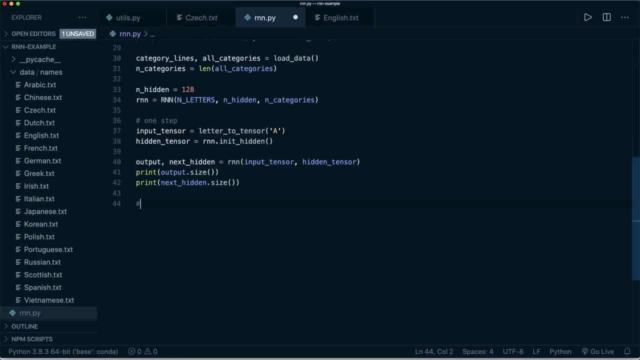 is what we want to do for one name. So now we say we have the whole see quence or the whole name, And here we say our input tensor equals, and then we use line to tensor and here, for example, we use the name Albert and then 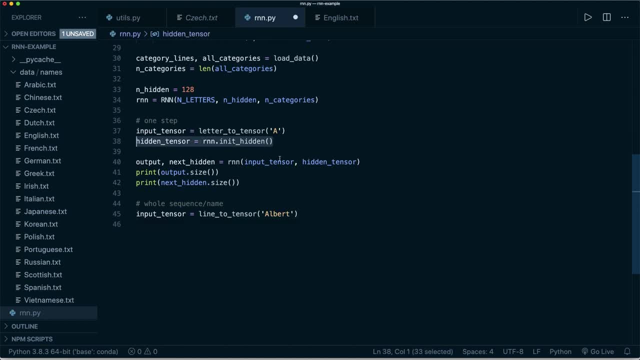 our hidden tensor is the same, And also this call is the same. So we grab this and copy this, And then here we use slicing, So we copy this, And then here we use slicing, So. So we only use the very first letter now for this simple example. So let's try this and 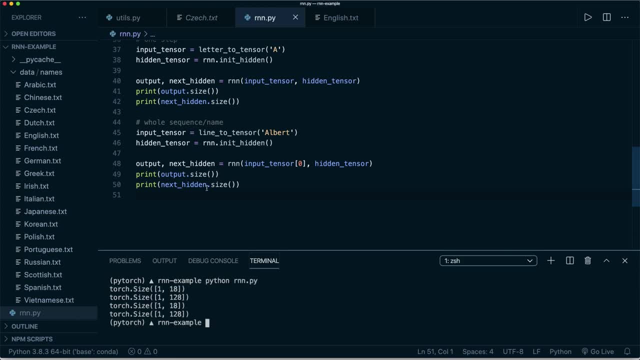 run it and see if this is working. So yeah, so this is working. And now here, what we have to do is we have to repeatedly apply these characters. So for this let's write some helper functions first. So let me comment on the print statements out again. So now, 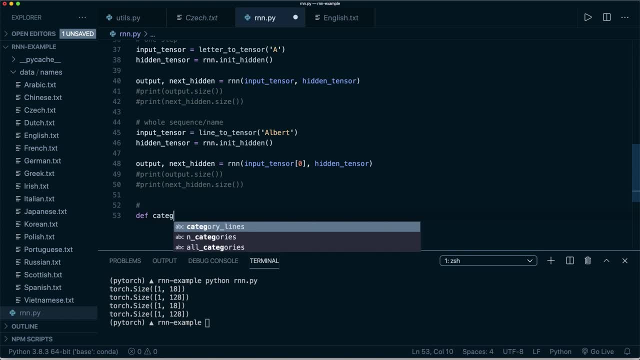 let's define a function And let's call this category to category from output, And this gets the output And, as I said, we applied the soft marks at the very end. So this is basically a likelihood of each character, of each category. So we want to return the index of the greatest. 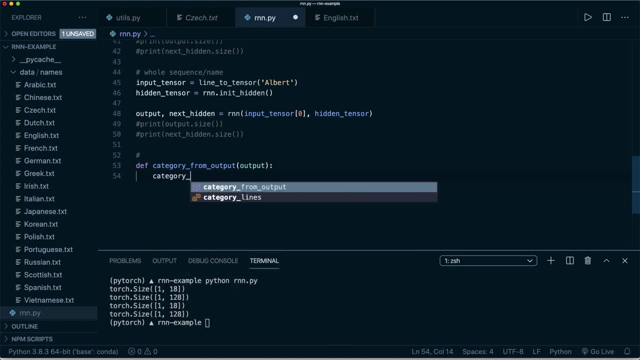 value. So we can get this. so category index equals, and here we can use torch, dot arc max, And then here we put in the output and then we can call the dot item, because this is only one value, And then we can return all categories, the 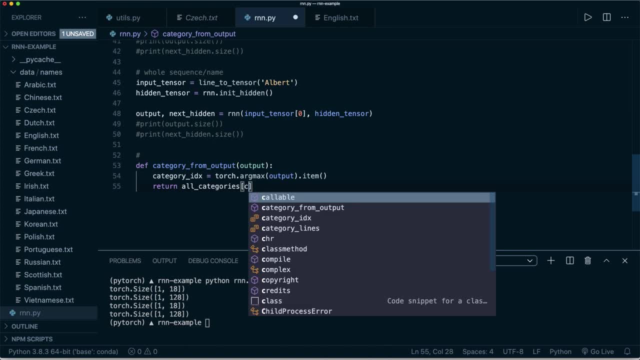 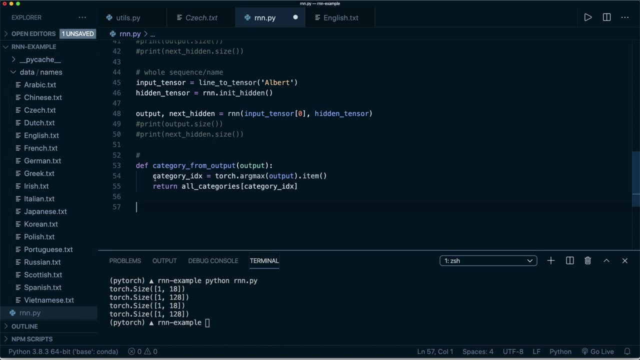 list with this index, category index. So this is one helper function. for example, now if we print the category from output and then here our output from this name, then if we run it, then we get: now this is Irish English and then we get our documents. OK, now we can run the report path from our library. And this is a huge part of JavaScriptום. now, for example, back in a night, make sure you, Then we get. now this is Irish and then we get some poggin, but we are running so much software Niceありò SATAR cl. sprayed out in the chat. So here we can see that with just this comma, sections. 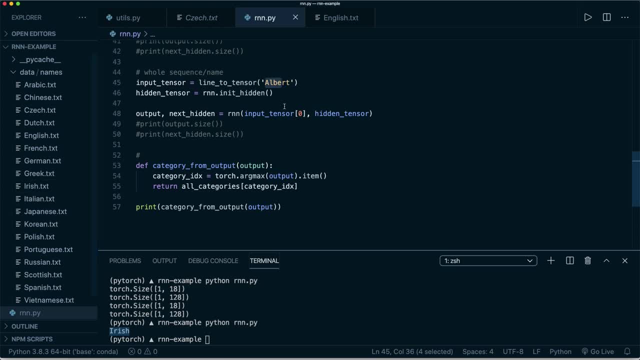 And, of course, this is not trained yet, So this doesn't look like an Irish name to me. So now what we want to do is we want to train our RNN, of course. So here, as always, we want to set up a. 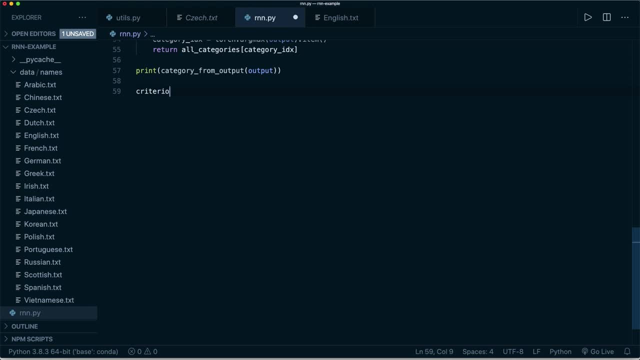 criterion and a optimizer. So we say criterion equals and here we use nnnll loss. This is the negative log likelihood loss. then we need to specify a learning rate, And here we have to be careful. So in this case I try point 005.. And the learning rate is very important here, So you might. 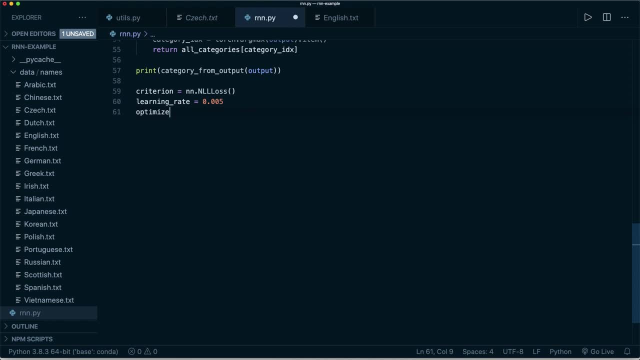 want to play around with this a little bit. And then we say our optimizer equals torch dot, optim dot SGD, So stochastic gradient descent. and then we want to optimize RNN dot per parameters And as a learning rate we use the defined learning rate. So now we have our loss and criterion And let's define another helper. 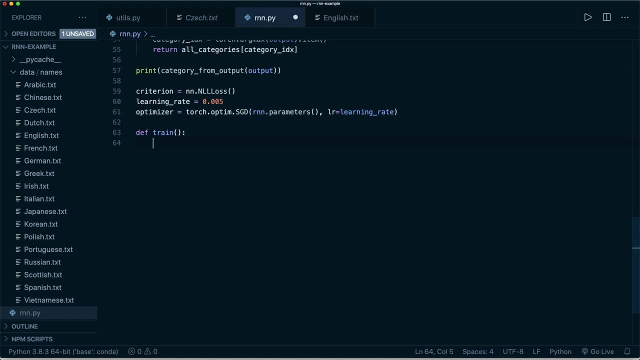 function and call this training. So this is going to be one training step And this gets a line tensor, So the whole name as a tensor, and it also gets the category category tensor. So this is the actual class label or the index of the class label. And now here we want to get a initial. 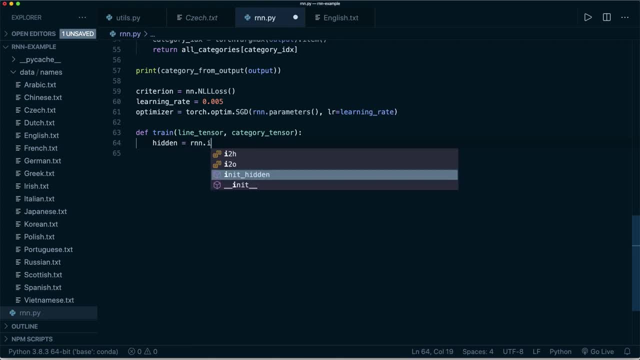 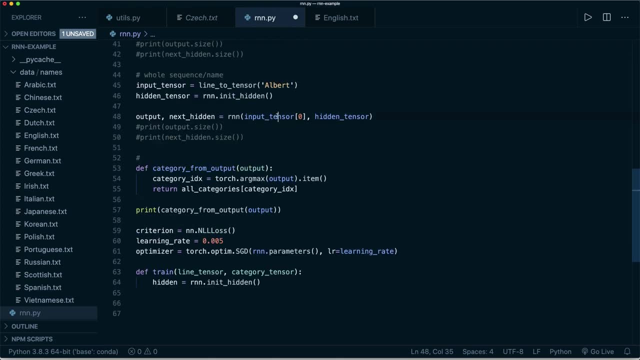 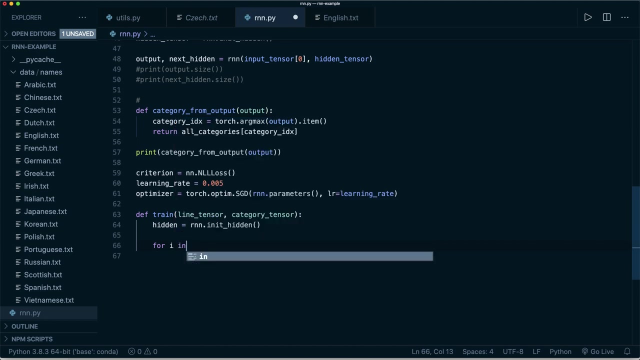 hidden state. So we say hidden equals RNN, dot init hidden. And then, as I said, we want to do this repeatedly, So we need a for loop. So we say for I in range and then the length of the line. 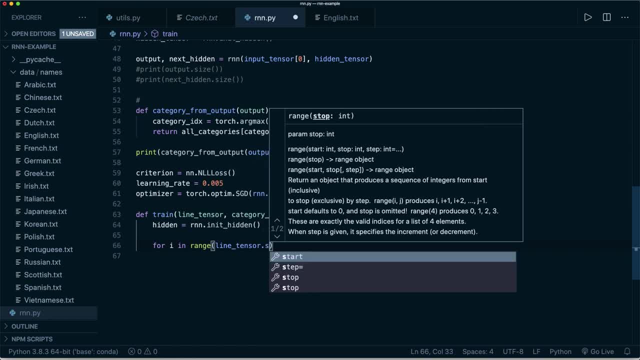 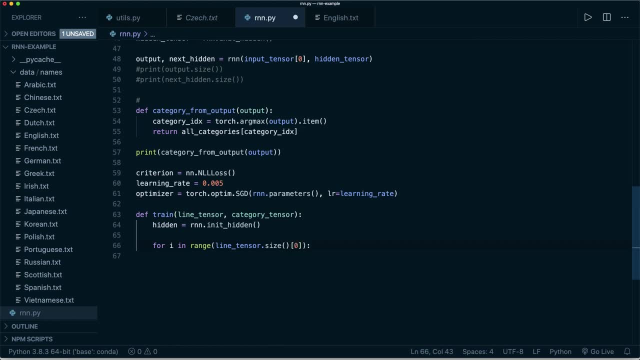 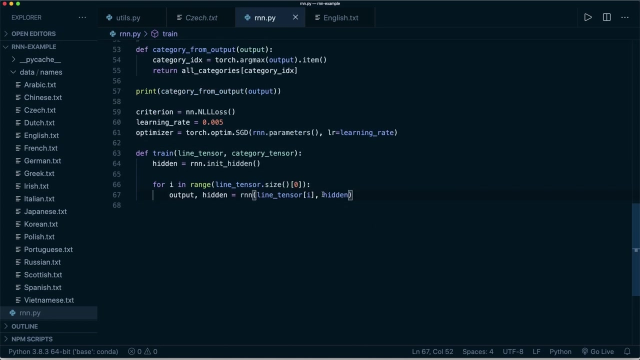 tensor. So we say line tensor, dot size and then index zero, So this is the length of the name basically, And then we apply this, So we say output and hidden equals RNN And it creates the new field. And then we do this for the layout. With the line tensor of the current index of the current character and the previous hidden state. So note that we put in the hidden state and then assign it also to the same variable. So the new hidden state will be the output from the RNN. 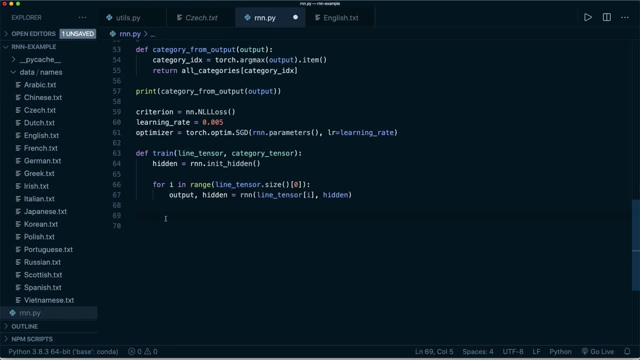 vector, we get the final output, And then we use this to calculate our loss. So we say: loss equals, here we apply our criterion with the output and the category tensor, And then, as always, we do our optimizer steps. So first we say: optimizer zero gradients, then we 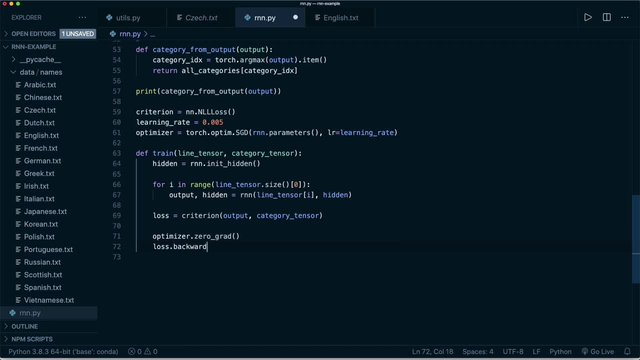 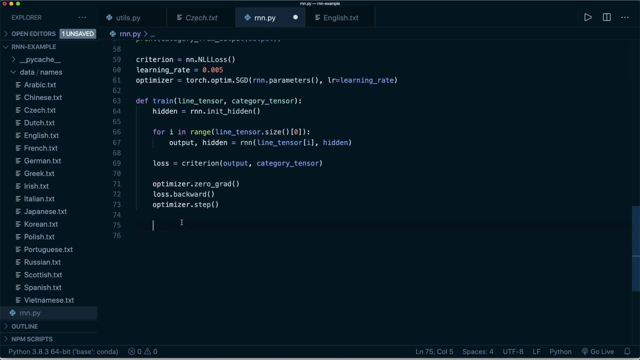 say loss dot back word, and then we say optimizer dot step, And then at the end of each training step let's return the output And let's also return the loss dot item, So not as tensor but as float value. And now we have this helper function for the training step. And now we 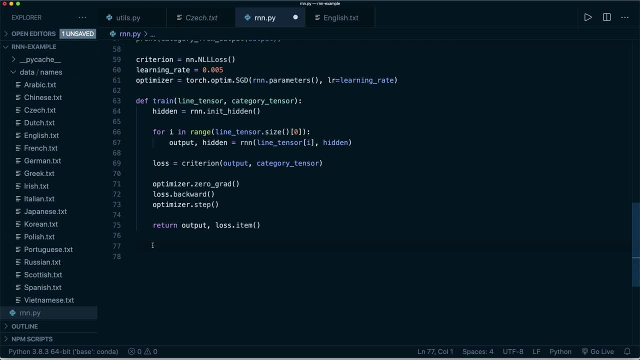 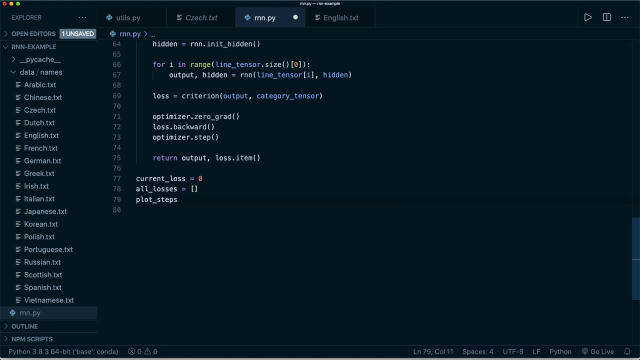 can do our typical, typical training loop. So for this let's track some things. So let's say the current loss equals zero in the beginning, then all losses equals an empty list. So here we want to put in all the losses so we can plot them later. Then let's say our plot steps and also our print steps equals. 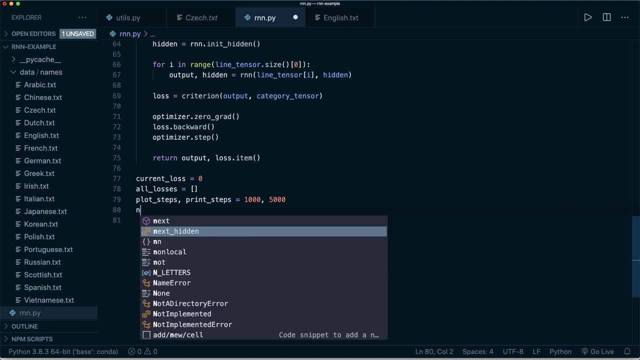 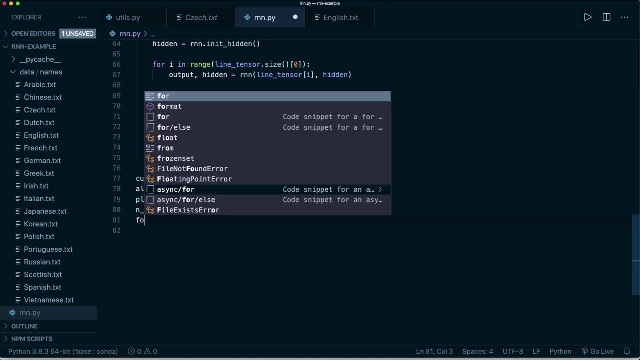 let's say 1000 and 5000. And the number of iterations equals, let's say, 100 style 1000.. And then we say, for I in range and hitters. And now what we want to do is we want to get a random training. 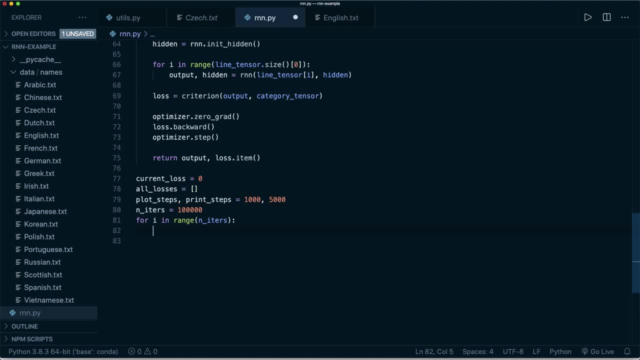 sample. So we have this as a helper function And this returns a, the category, then it returns the actual line or the name, Then the category s tensor and also the line s tensor. And we get this by calling the random training example function from the utility class, And this needs the category lines as 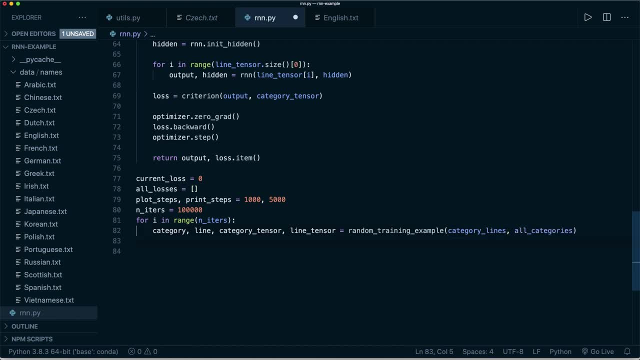 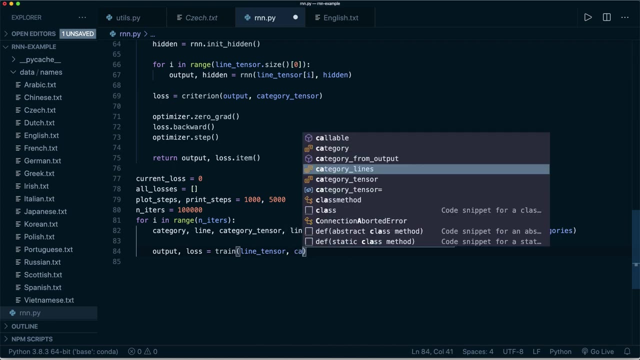 input and all categories And then we call the training function. So we say: output and loss equals training And this gets the line tensor and it gets the category tensor. then we add the loss to our current loss, So we say current loss plus equals loss. And then we want to: 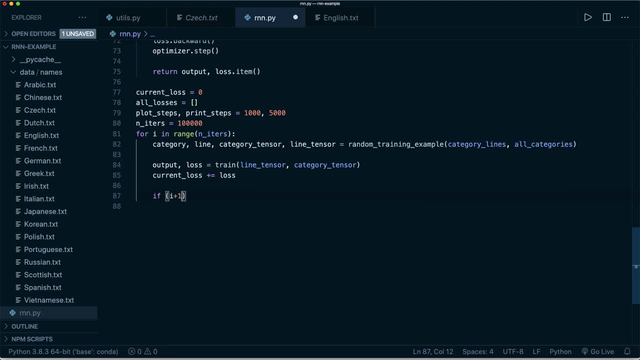 print some information. So we say: if I plus one module or plot steps, so every thousand step if this equals Zero. so here we want to calculate the current running loss and append it to all losses. So we say: all losses, dot append, and here we say current loss divided by the number. 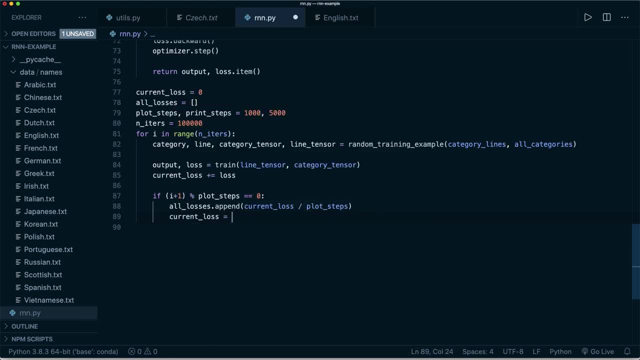 of plot steps, and then we set our current loss back to zero, because here we added up for every iteration and then only every thousand step we append it, So we have to divide it by the number number and then we get the average. And now we do the same with the print steps. So we 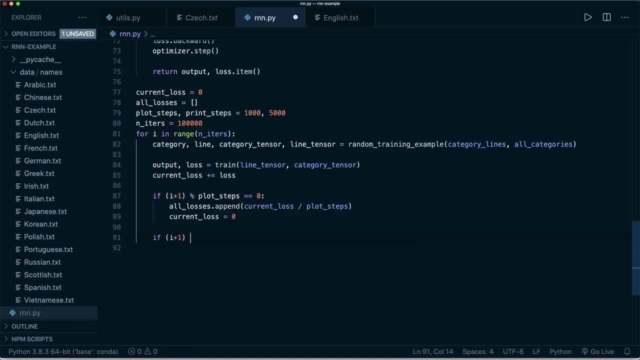 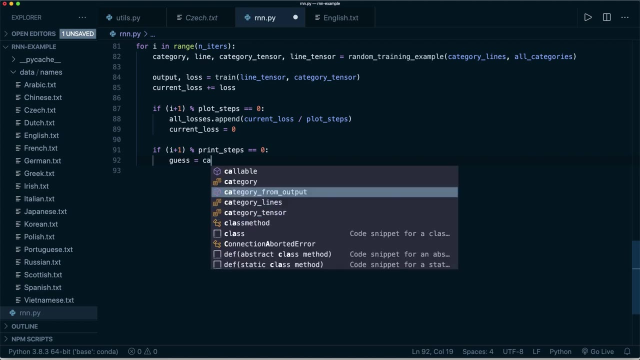 say if I plus one modulo print steps equals equals zero. then we want some it print some information. So first we want to get the guests. So we say guests equals category from output And we put in the output of course. then we check if this is correct. So we say 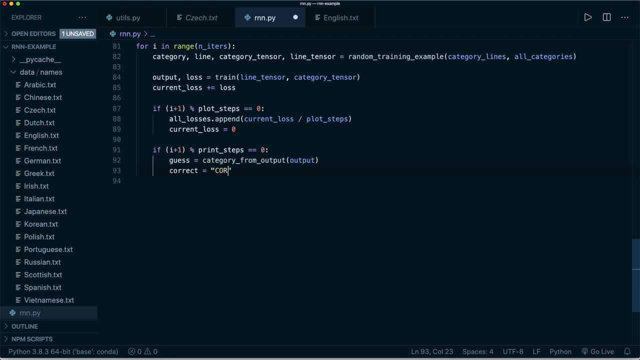 correct equals, and then we say correct And this is correct If the guests equals, equals the actual category that we get from the random training example. And if this is not correct, then we print print wrong And we also want to print the actual categories. So let's use this as an 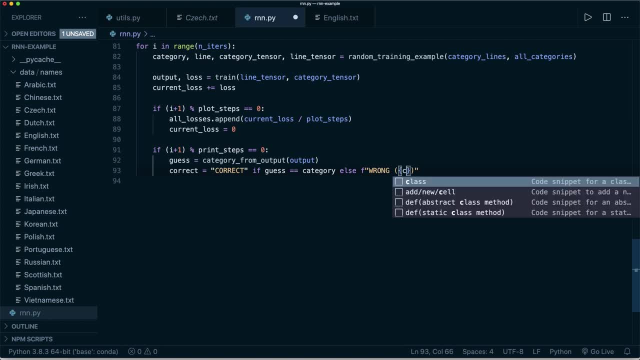 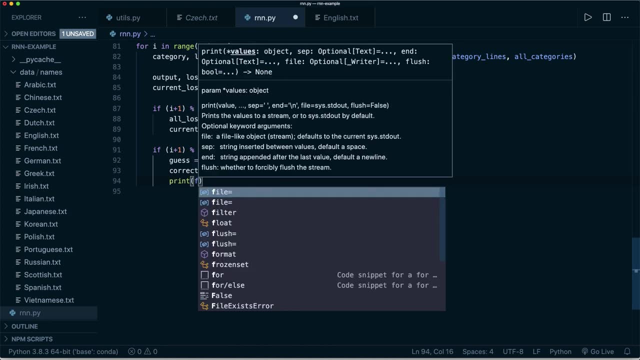 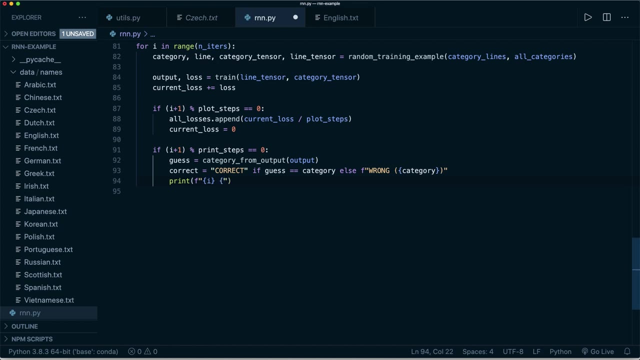 F string here And here let's print the actual category And then we print as an F string. Again, we want to print the current iteration step. Then we also let's print I divided by the number of errors times 100.. Then let's also print the current loss. So we say loss and let's 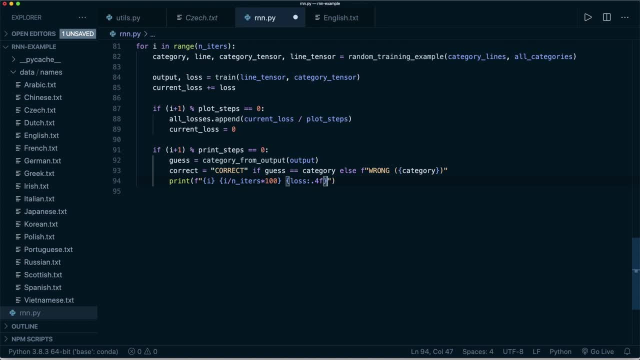 print only four decimal values And let's also print the current line. So basically, this is the name, And then let's print the guests, And let's also print the if it's correct or not, And now we are done. So this is basically all that we need. And now, when we are done, 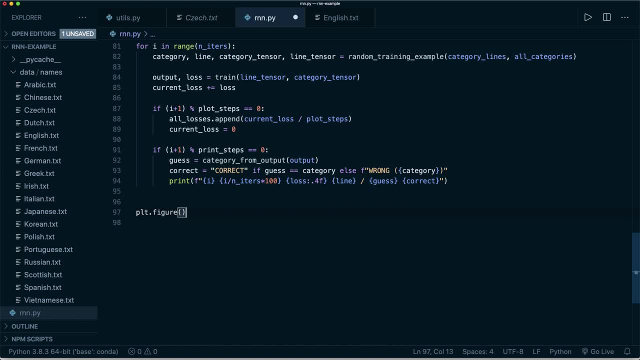 let's plot our losses. So let's create a figure with Matplotlib, So PLD nut figure and PLT dot plot. And here we want to plot all the losses and then say: plot show. And now we could already start our training. And now what? 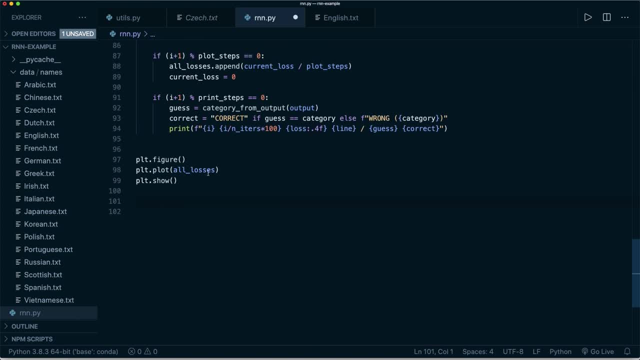 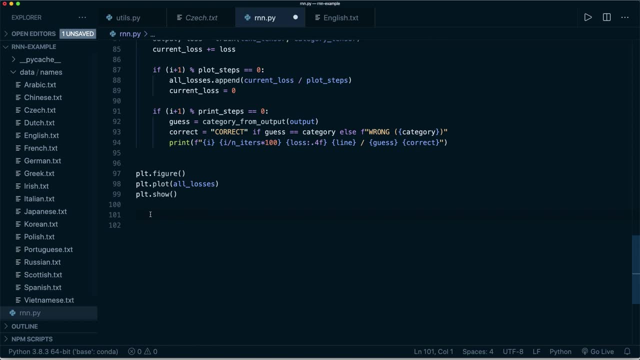 We're going to start a learning course, We're going to start a more onesign activity, And then we, for example, what we can do is we can save our model here and then use it later or for for whatever we want, But in this case I simply want to try it myself. So I say, while 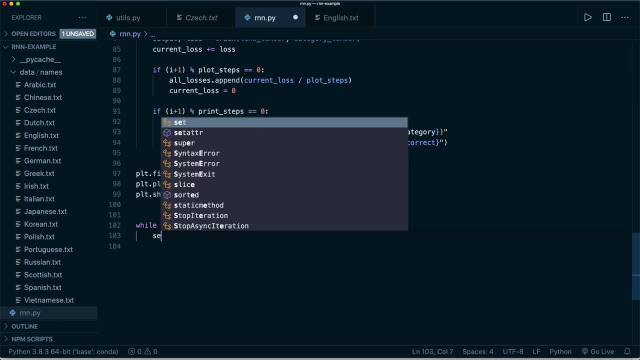 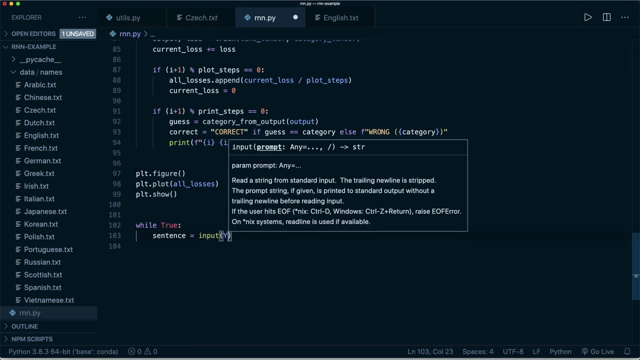 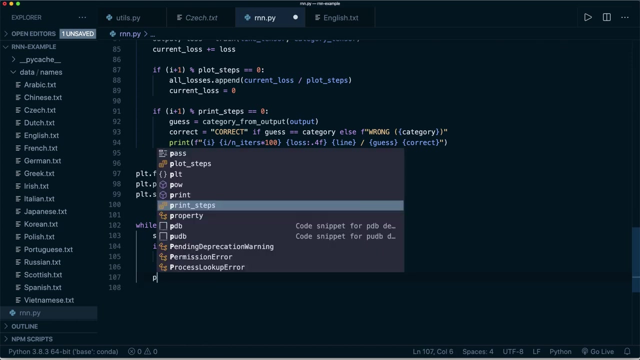 true. and then I say I get an sentence as input, and let's say input, And then I put this to a function. Or I first let's say: if sentence equals equals quit, then I break, and otherwise I want to predict the sentence. So for this let's create another little helper function. 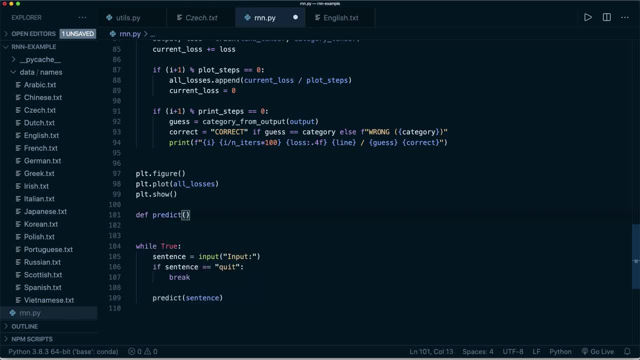 Let's call this predict, And this gets the input line So as raw text. So first of all I print, Let's print a new line, And then let's print the input line as well. So for this, of course, we need an F string. And now, here in our prediction, we should: 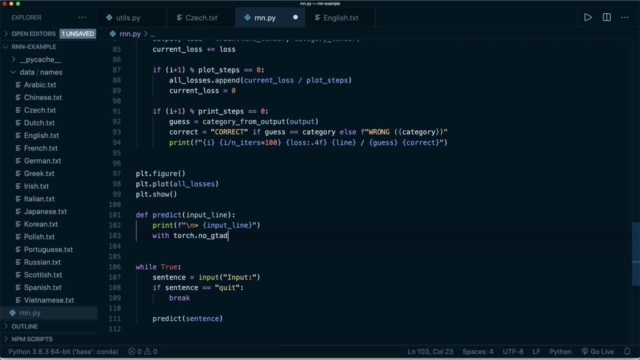 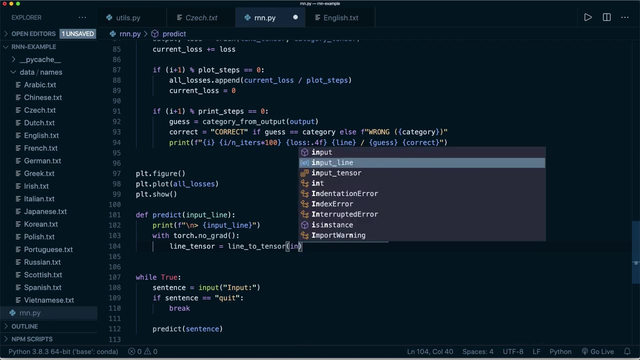 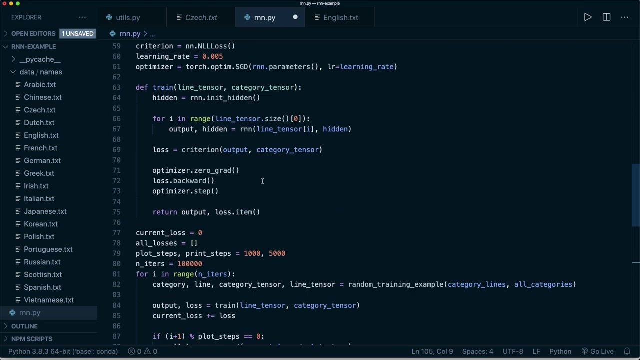 use torch dot no grad So we can turn off the gradients now. And then what we want to do is we want to say our line tensor equals line to tensor from the raw input line, And now we want to do the same as we're doing in our training step. So you have the initial hidden states and 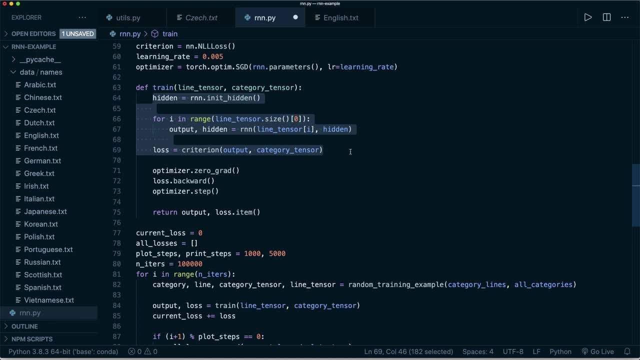 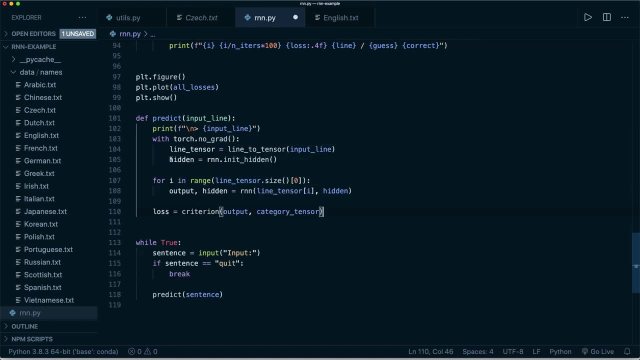 then repeatedly apply our RNN, And let's do this, So let me copy this and put it here, So we have the initial hidden state. then we say for I in line tensor size zero, So, and then we get the new output and the new 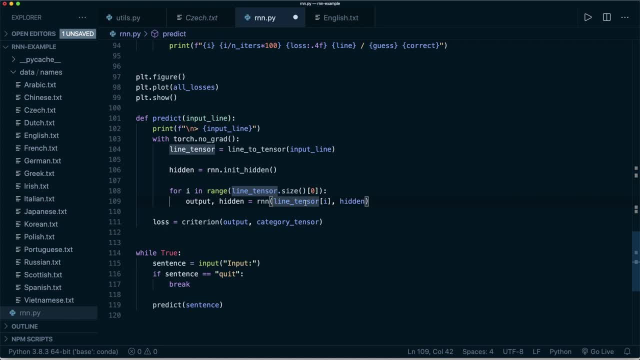 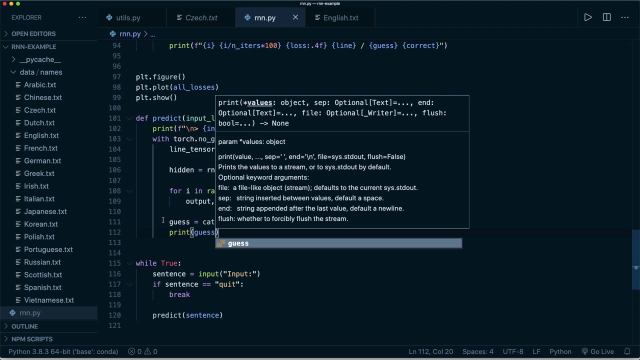 hidden state by applying the RNN, And then at the very end we want to get the guess. So we say guess equals, and then we say category from output and we use the last output from the last step And then we simply want to print the guess here. So in this example, 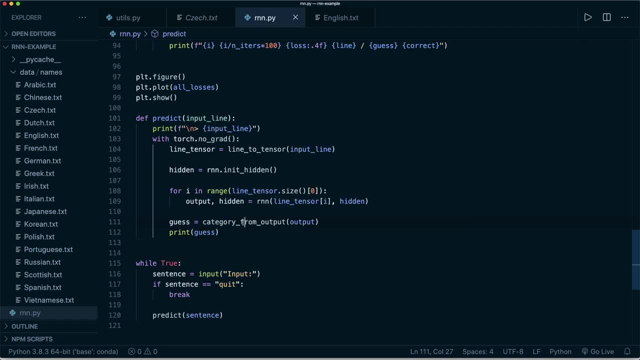 I don't calculate the accuracy or anything, I just print the guess and see if it's correct or not, So yeah, so let's save this And let's run this and hope that everything is working. So this might take a few seconds or minutes. So this is from. 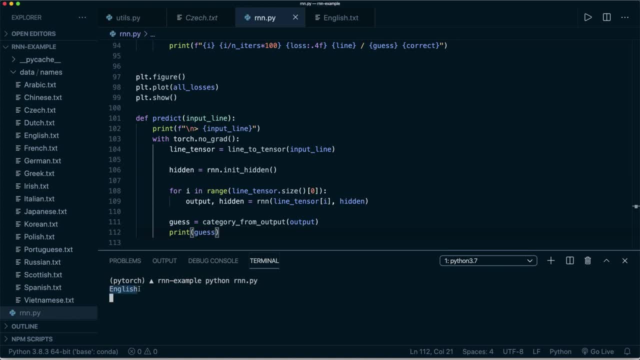 the first example that I showed you. And now we see we have step on. this should be 5000. And this should be 5% of the training is done. And then we have the loss and we have the name and we see that the guess is wrong because this is actually polish. 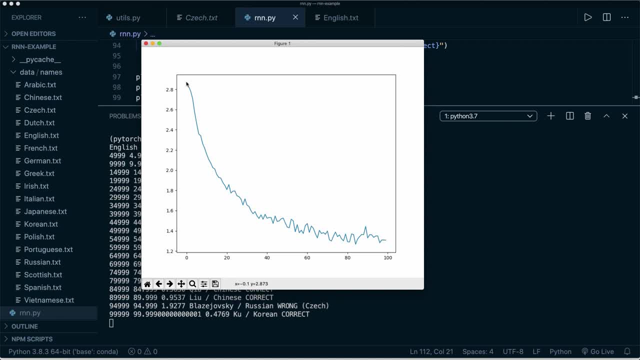 All right. so now it's done and it's plotting the losses and you see that it's decreasing very quickly. and then it's trying or jumping around a little bit, but still decreasing. I think this is a pretty good result. So let's have a look at some random guesses during the. 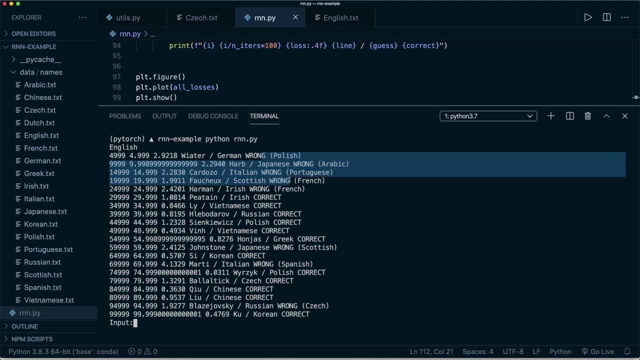 training. So we see that in the beginning almost every guess is wrong, And then it's starting to learn some things. So now it's starting to do correct predictions, But of course it's still not perfect, So there are still wrong corrections. But yeah, at the very end we have this loss. 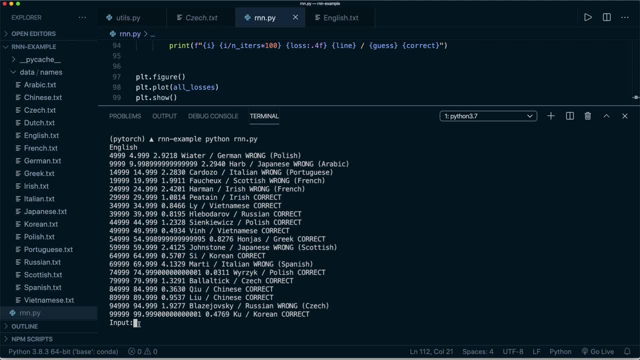 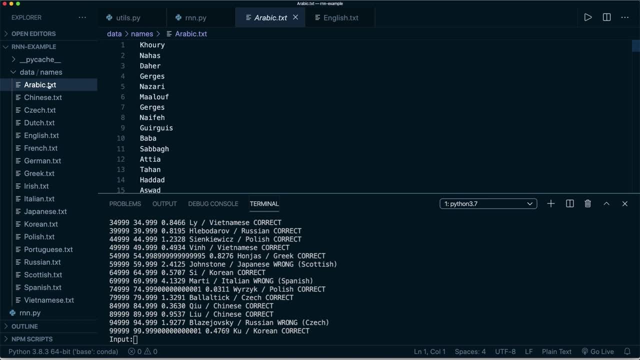 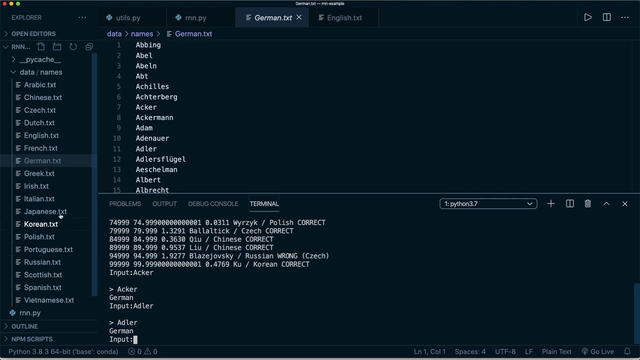 so this is pretty good And now we can try it ourselves. So now, for example, we could go and try some names from those files. So, for example, let's start with some German names. So let's try occur, And we see it says German. So let's try Adler, for example, And 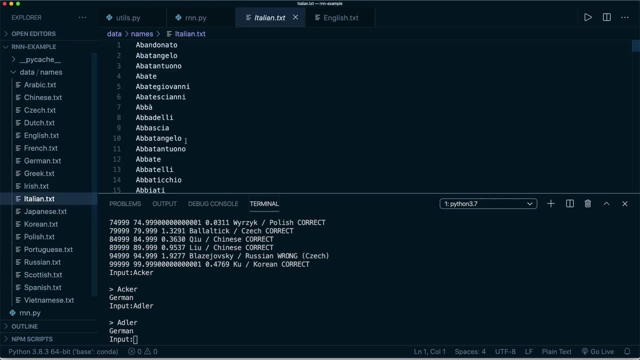 this is also correct. So let's try some Italian names. I think these are pretty clear to detect. So let's try about Delhi, And it says Italian. So this is correct. So let's try some Russian. for example, let's say a buy him off, And it says Russian. 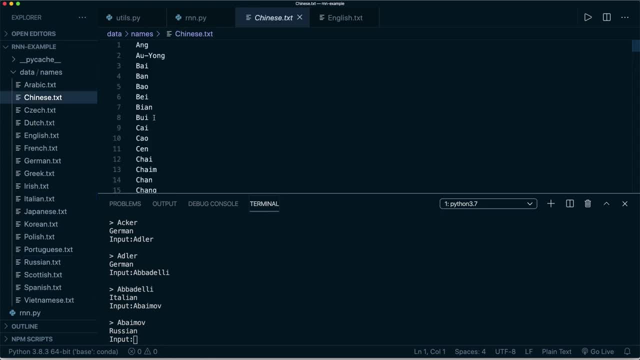 Yeah, great. So let's try something more difficult. for example Chinese. So let's try bow, And it says correct, Wow, let's try by- still Chinese, So it looks like it's. it's working pretty nice in this example. Of course, it's still not perfect. 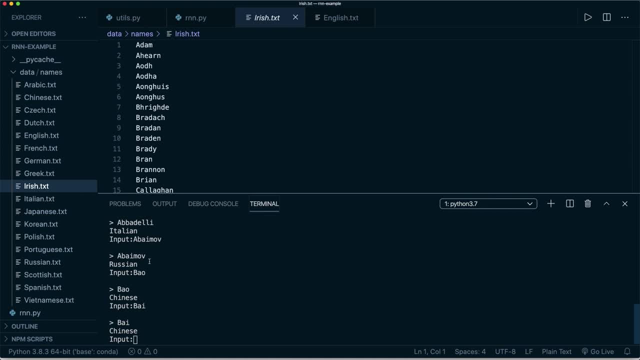 But for now all the guesses are correct. So now you see how we can train a RNN to do name classification And, yeah, I hope you enjoyed this tutorial And now know how RNNs can be implemented in pytorch. If you liked this tutorial, then please consider subscribing. 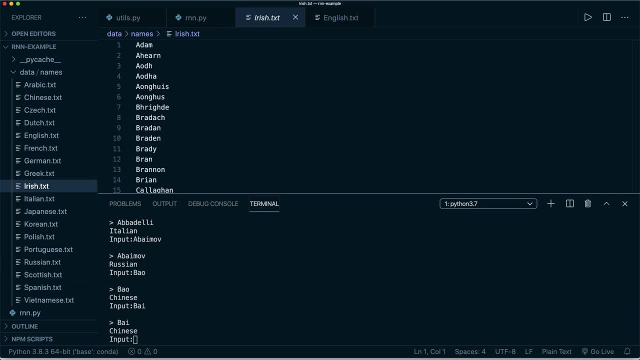 to the channel and leave me a like, and see you next time. Bye.